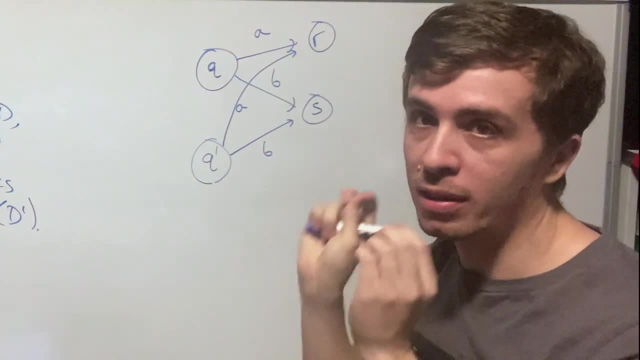 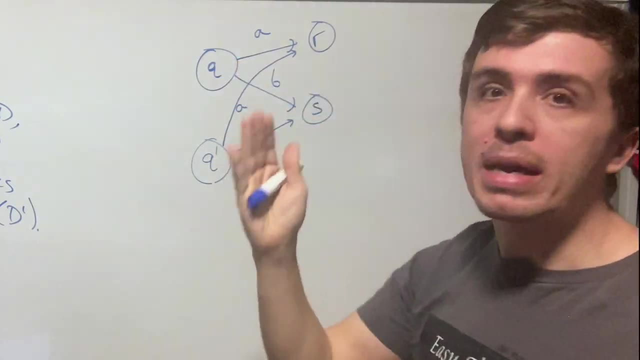 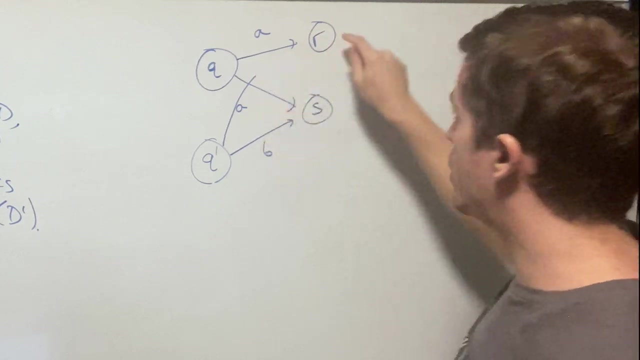 state And then, therefore, because these states are literally doing the same thing and the fact that they're both not accepting, then we can merge these two states together And we can actually generalize this a little bit further. So what if, for example, we had- let's just notice that R and S are not accepting either? 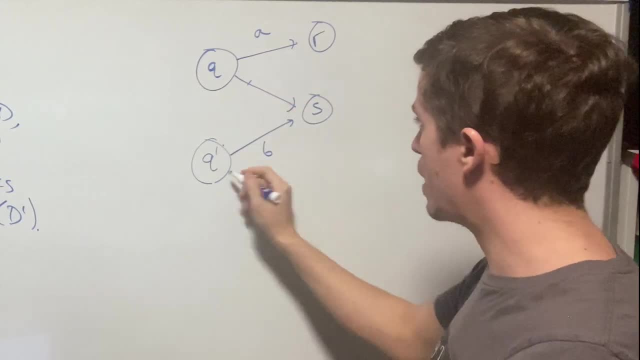 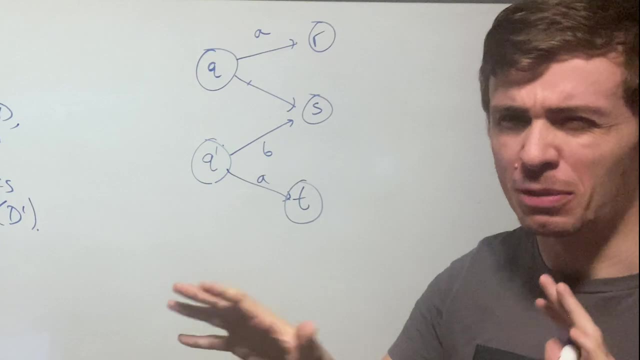 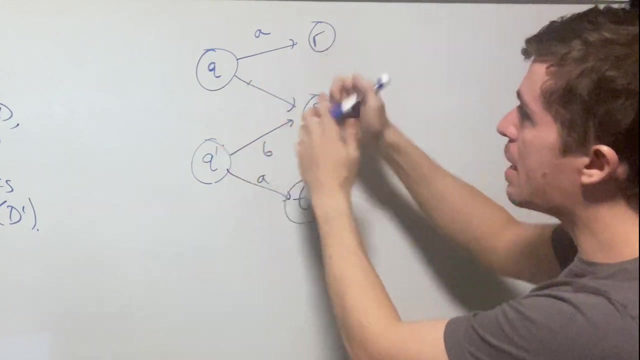 Well, what if this A transition went to another state? let's call it T. that is also not accepting, And we would have to guarantee some other things too, but let's set that aside. So note that the A transition goes to a non-accept state and the B I erased it. 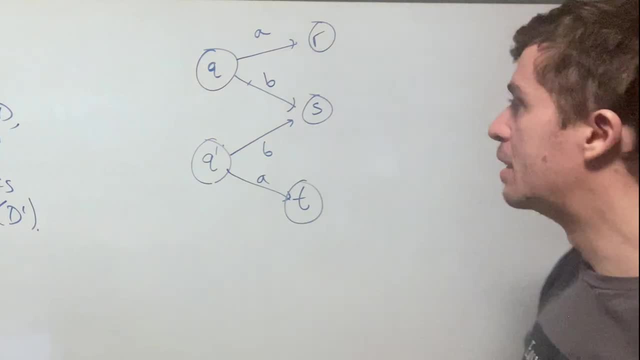 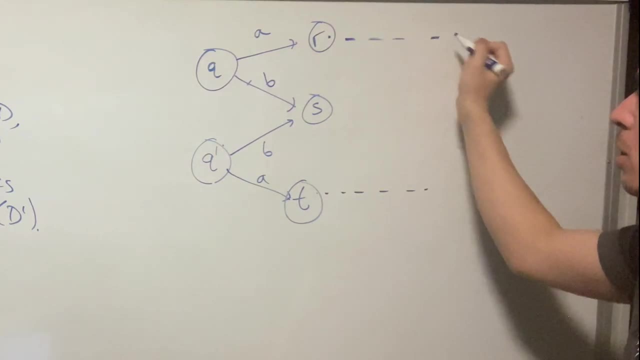 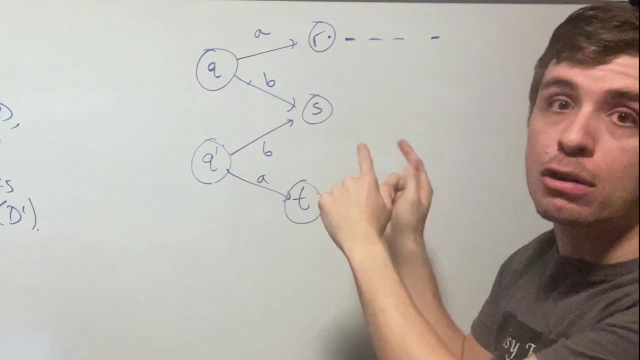 B transition goes to the same state in this particular case. So then we would have to guarantee something else about what happens after the T and the R states. If they go to exactly the same state, then obviously anything that appears after would be identical for both states. Q and. 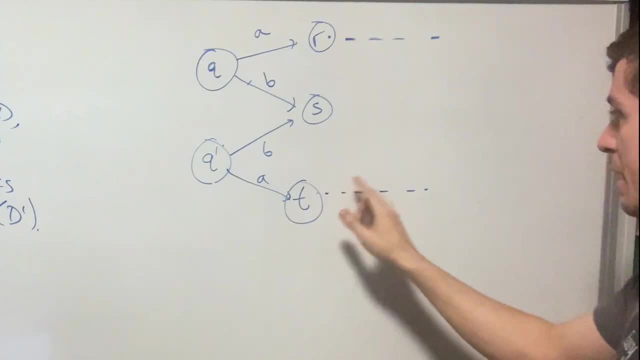 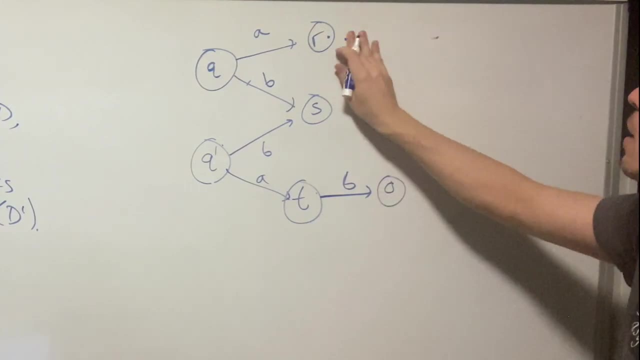 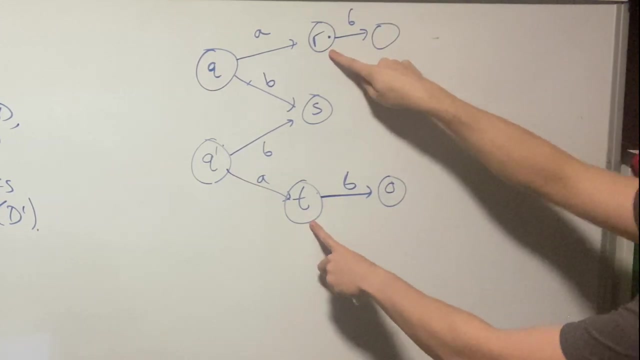 Q prime, because they're literally going to the same state, Whereas here, what if, for example, B on this state goes to some accept state and then a B on this state goes to a non-accept state? Then that means that these two states are. 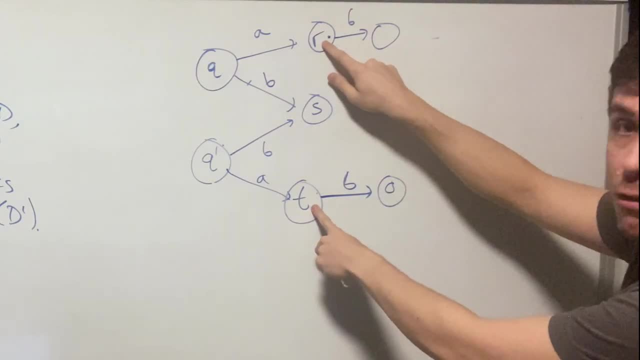 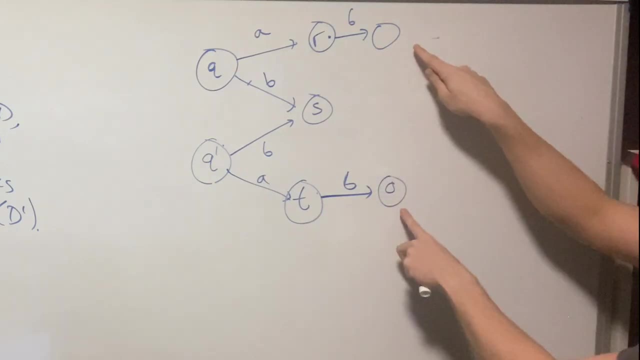 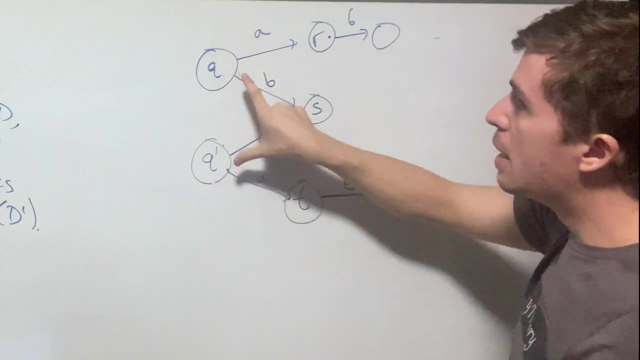 not equivalent at all, Because if you read a, B from them, you're going to, in one case, accept and not accept, and in the other case. So then therefore, in that case, if we're in here, we can say that Q and Q prime are not equivalent, Because if they were, then that means reading any. 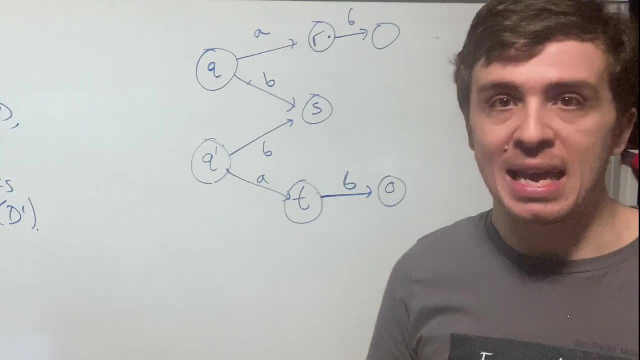 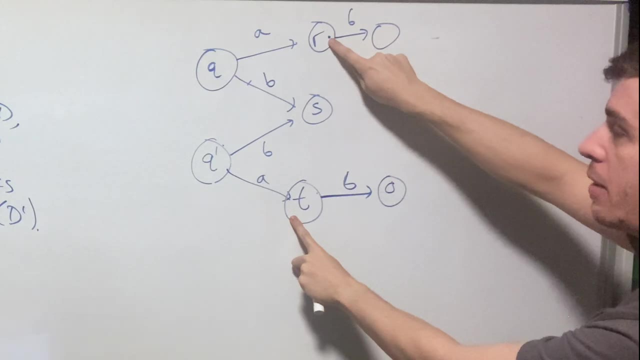 string at all will always result in a non-accept state. So if you read a B from them, you're going to in the same answer of whether to accept or not. So if we read a B in this case, we would follow the A transition and then the B transition and, oops, we accept in one case and not in the other. 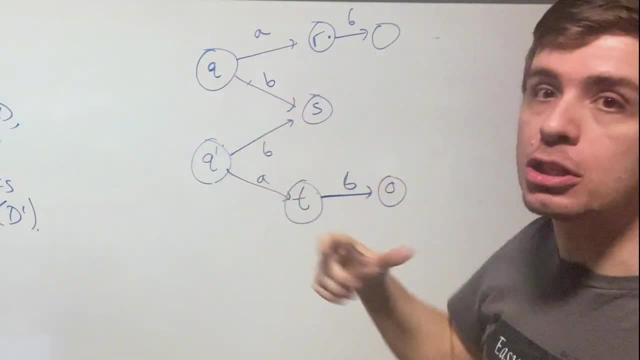 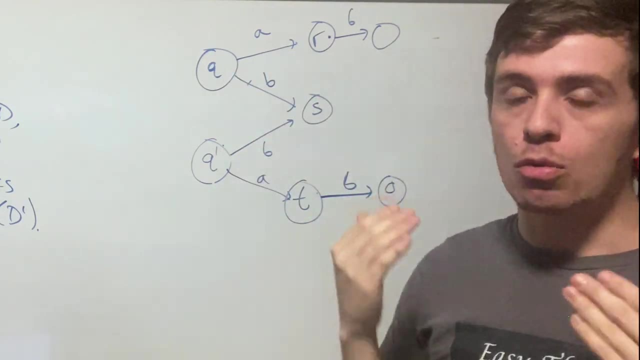 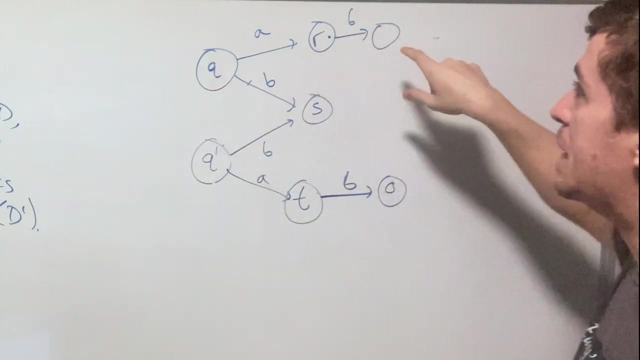 case. So that's what it means for two states to be equivalent. We're saying equivalent meaning that if you read any string at all, you will be either in the language both times or not in the language both times. It's not like this, where you're going to read a string at all and then 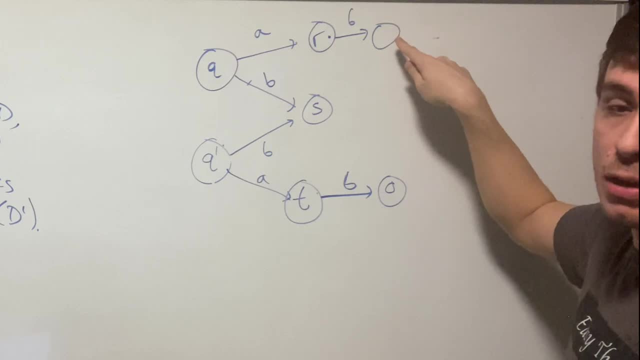 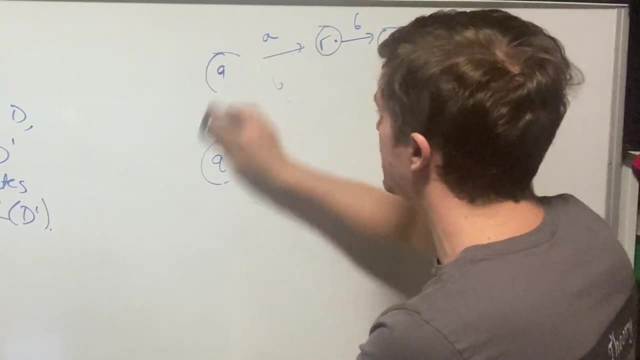 you end up in the language in one case and not in the language in the other. So now let's talk about the general whole DFA. So we're looking at a piece of the DFA, but let's look at a whole DFA. So let's. 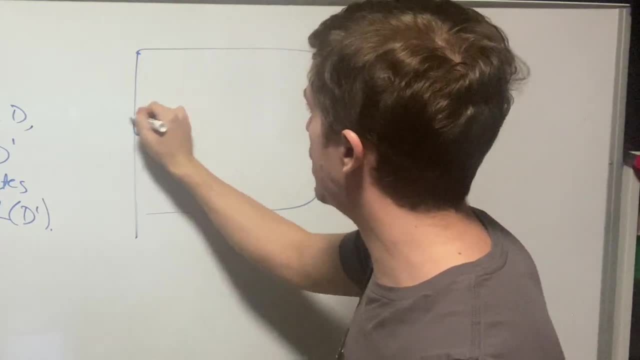 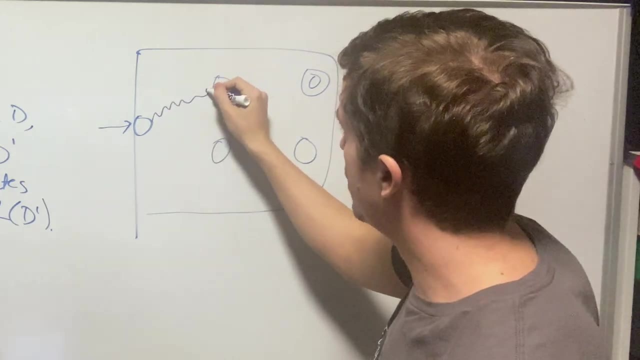 draw a particular DFA right here. So here's its start state, and then let's have some other states in here, just some random other states. Let's look at two particular strings in here. So I'm going to call this X and then I'm going to call this one Y. These can be obviously are two different. 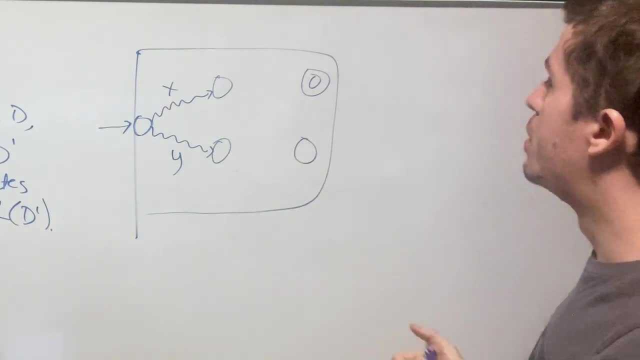 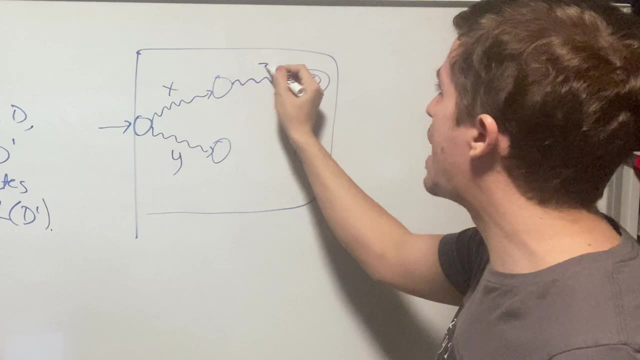 strings because they lead to different states, Because it's the same string, it's the same DFA. So now let's examine what happens afterward. So let's say that we read exactly the same string. after we read the X thing and then the Y thing, Let's say, just as a picture. just as a picture. 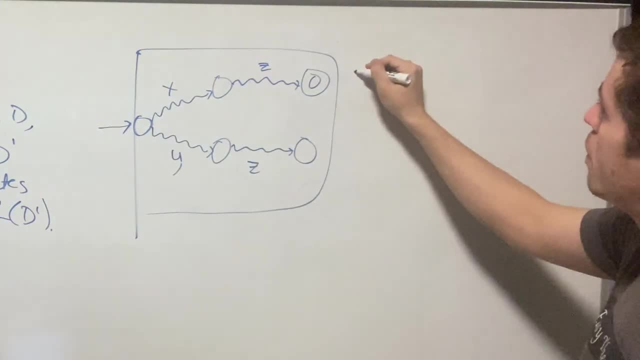 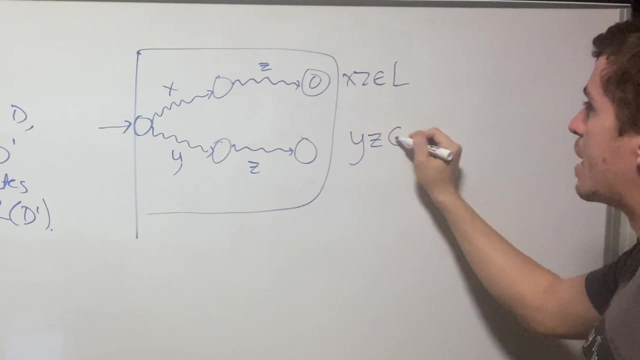 Starting the start state, read the X and read the Z. So then, therefore, XZ is in the language of this particular DFA and YZ is not in the language of this particular DFA. So then, therefore, the Z suffix. notice that there's a suffix in both cases. that is exactly the same. So that means. 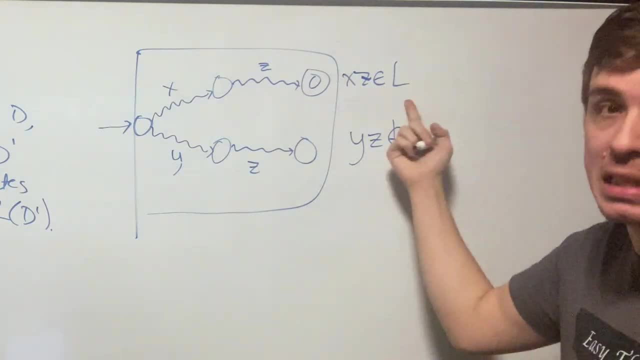 that X and Y are not equivalent with respect to this language. They individually. they might not both be accepted, and that's totally fine. Actually, if that was the case, then Z could be the empty string, if X and if one of these was accepted and one was not, But if they're both. 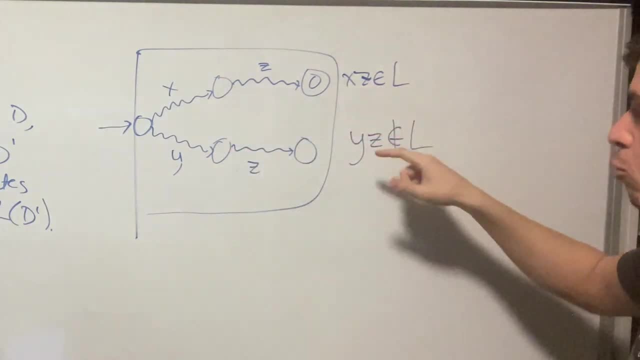 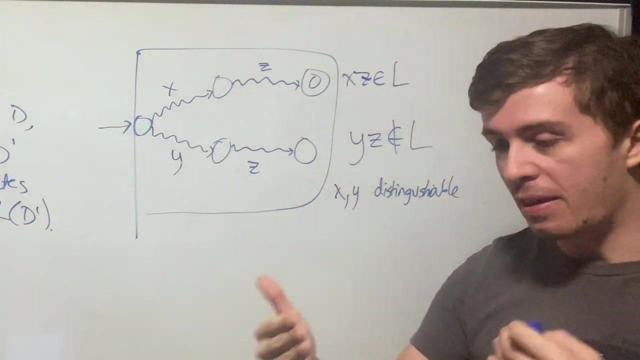 the exact same and we have the property that reading something else afterward will give you being in the language in one case and not in the other case. then we say that X and Y are distinguishable. So distinguishability just means that if you read that particular string, 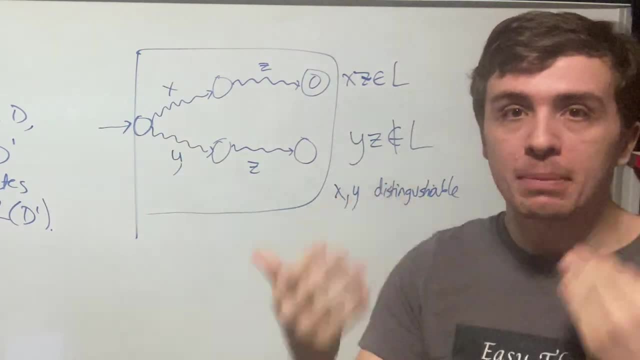 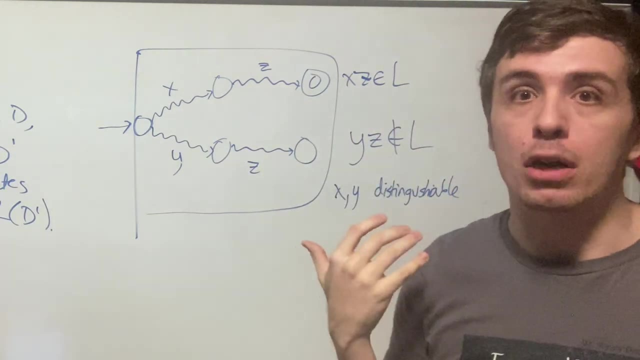 actually both of those strings, starting from the start, state there's some string afterward that eventually will give you differing answers. So then, if we have two strings that are indistinguishable, let's look at what that would look like. So then, indistinguishable means that 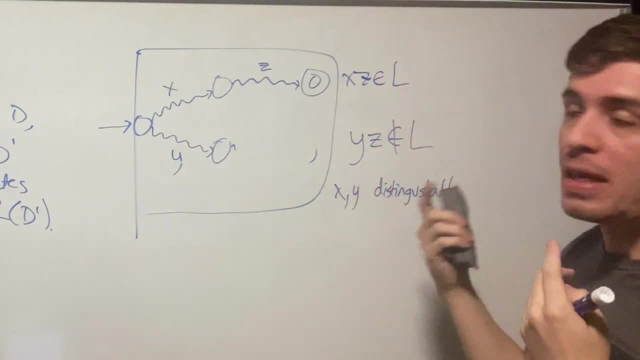 there is no difference between the two strings. So then, if we have two strings that are indistinguishable, there's no string that you can read afterward that will have differing answers. It's always the same answer every single time. If they're indistinguishable reading. let's say: 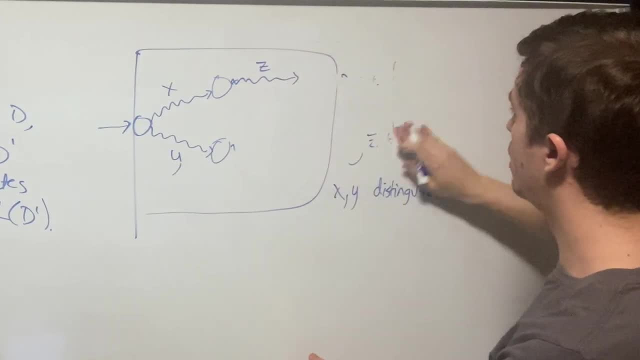 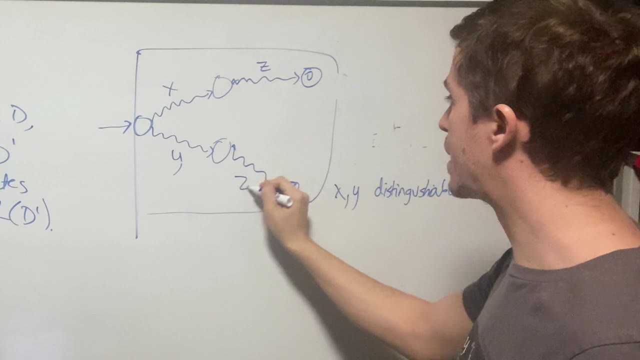 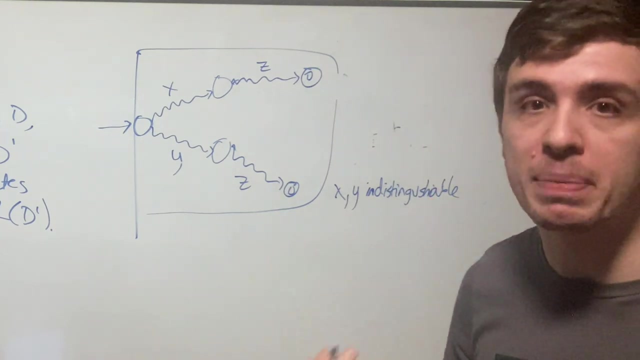 a Z afterward. so this doesn't apply anymore. reading a Z afterward will have, let's say it'll accept here, then it also must accept here, because we're assuming that these two strings are indistinguishable. They are identical with respect to the language. They might not be. 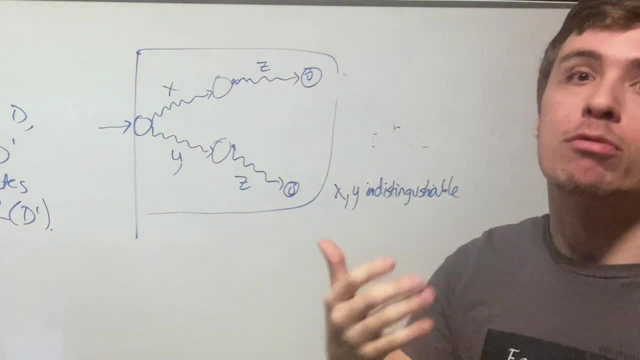 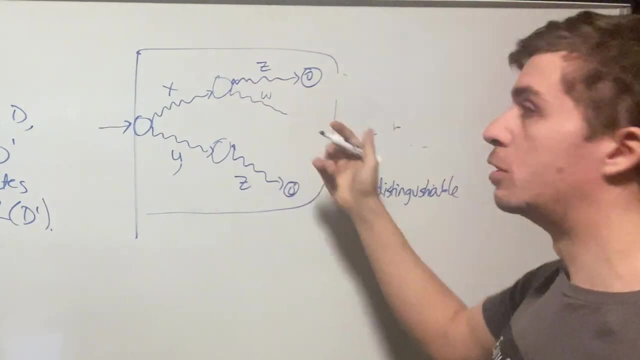 identical strings, but they're indistinguishable. So if we have two strings that are indistinguishable, obviously, but they're identical with respect to the language in terms of reading stuff afterward, But also what we can do is we could, we could read a particular string, suffix here. 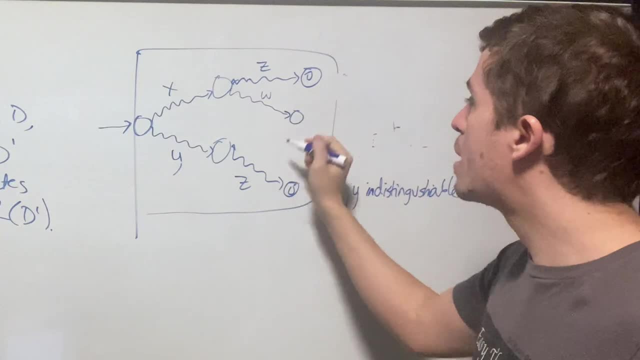 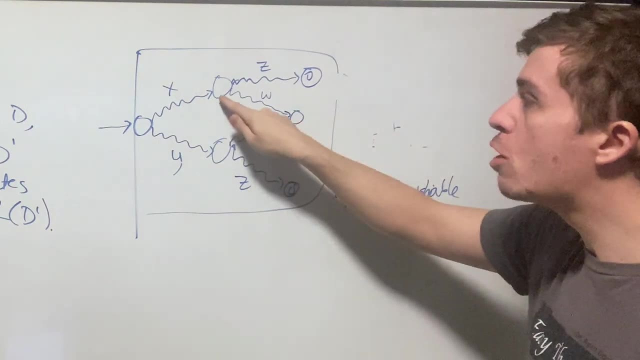 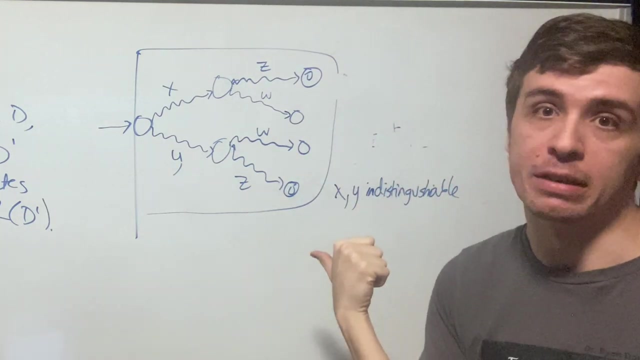 let's say W, and then that will, let's say, go to a not accept state, And then maybe this one also goes to a not accept state. So if it's the case that anything you read after X or Y will always give the same answer, then they're indistinguishable. That's what indistinguishability. 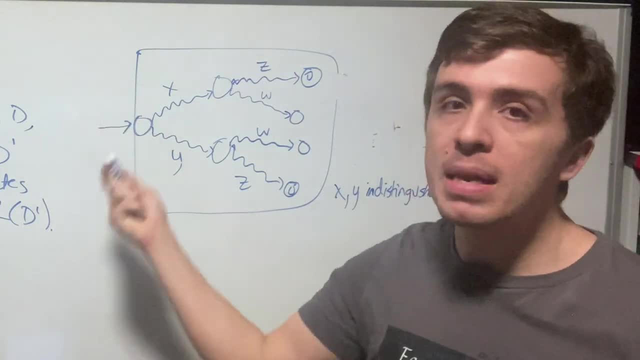 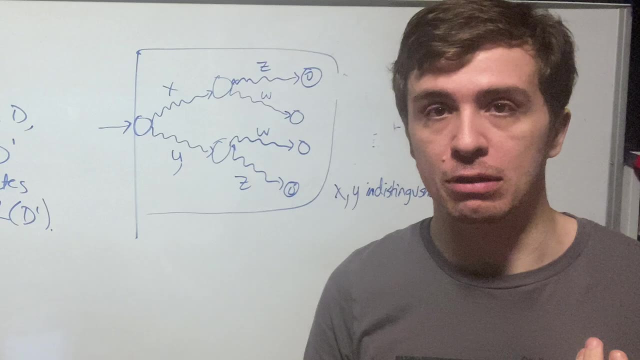 means. So if you have two strings that are indistinguishable, then they're indistinguishable. So actually, the whole algorithm for minimizing a DFA is determining what states are distinguishable and what states are indistinguishable. All that, a distinguishable? 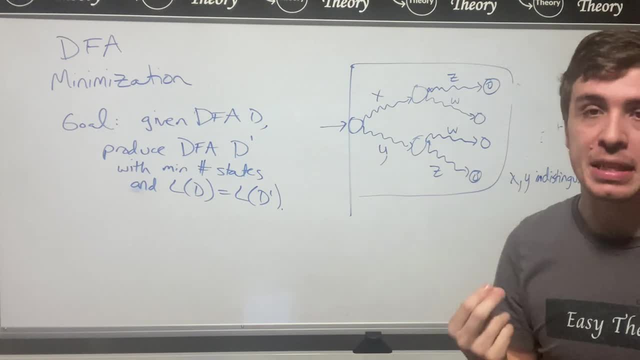 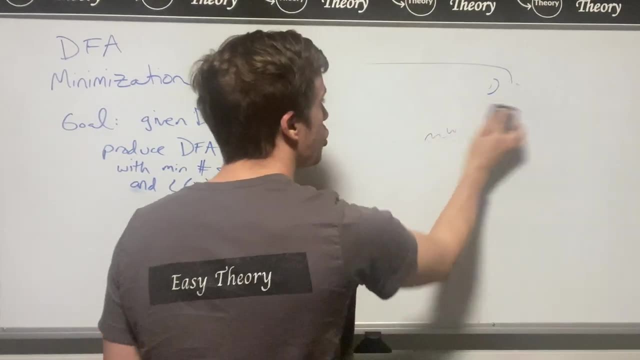 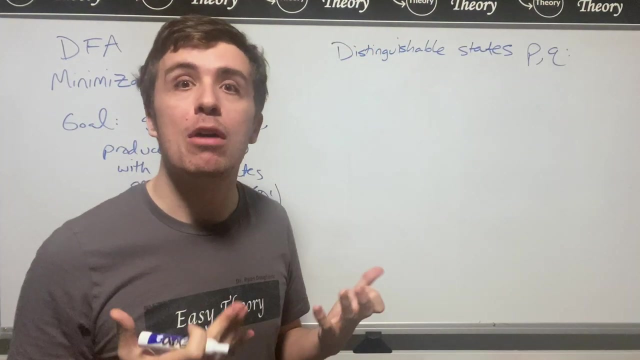 state means it's slightly different than a string, but distinguishable states are one of three different categories And it's actually going to lead right to the algorithm And it's really really easy. So what is a distinguishable state? So let's try to figure out what a distinguishable 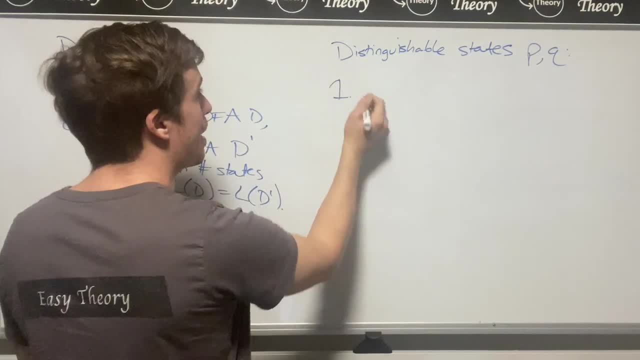 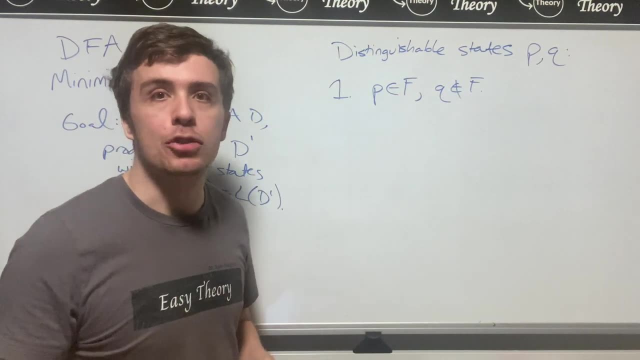 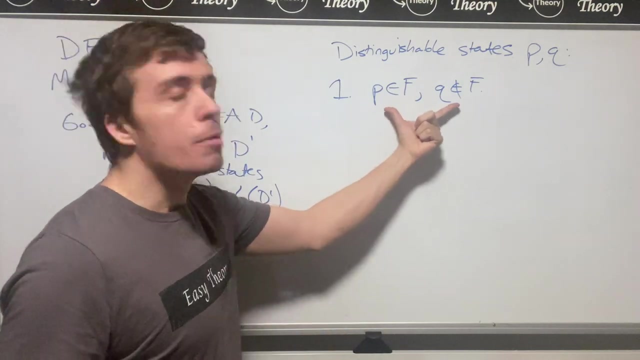 state is. Let's try to figure out whether P and Q are distinguishable states. One case might be that P is a final state and Q is not a final state. If we read any string afterward, if they were indistinguishable, then the answers would always be the same. But it's not here because we can. 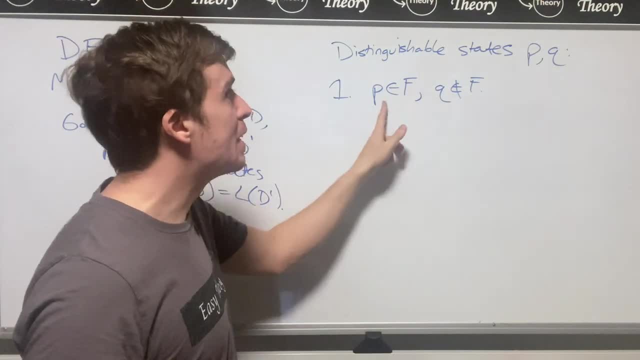 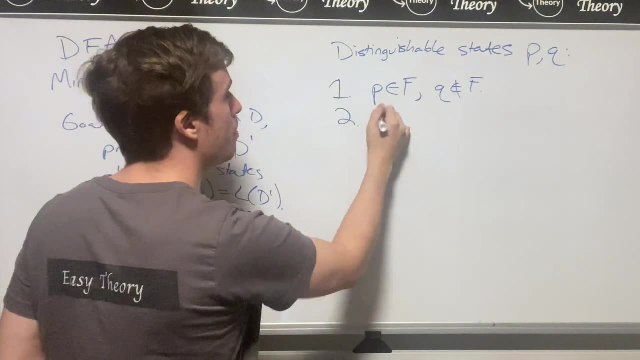 consider the empty string. If we read the empty string from either one of these states, then one of them is a final state and one of them is not a final state. So the second case is just flip this around. It could be that P is a final state and Q is not a final state. So let's try to figure out. 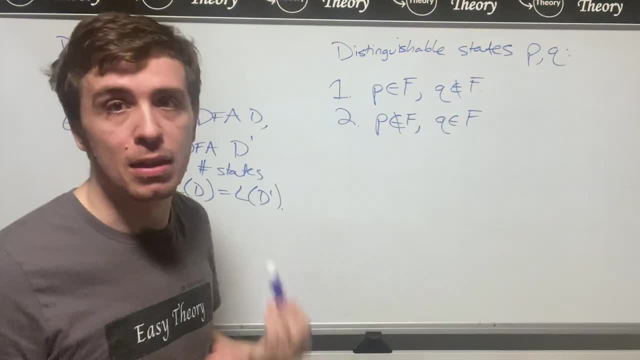 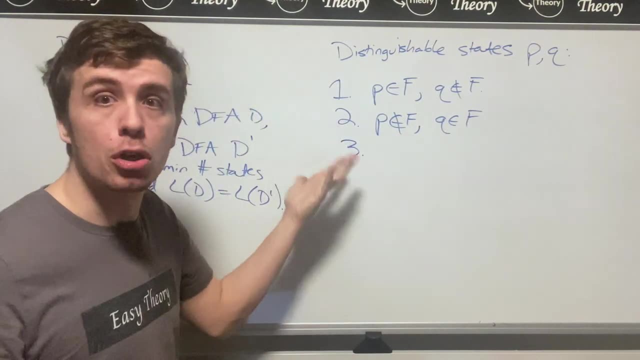 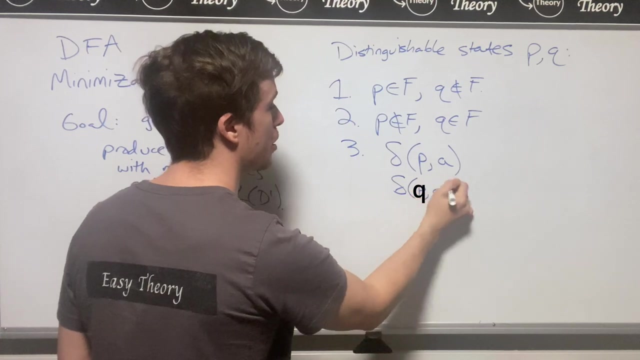 that P is not a final state and Q is a final state, And that logic obviously follows. So then the third case is what we call the recursive case, So you can actually define this recursively. So let's look at the transition function from both of the states on a particular character. So let's 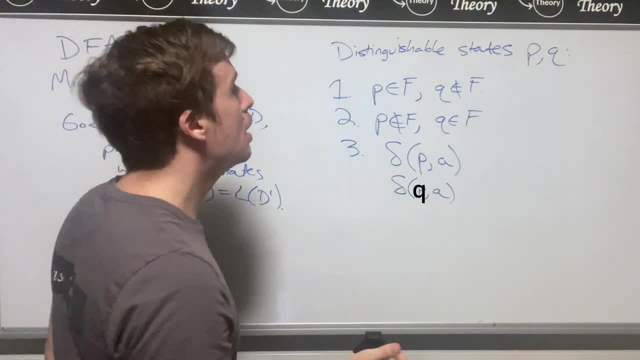 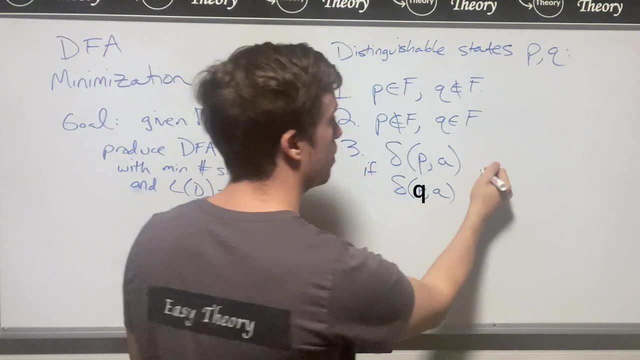 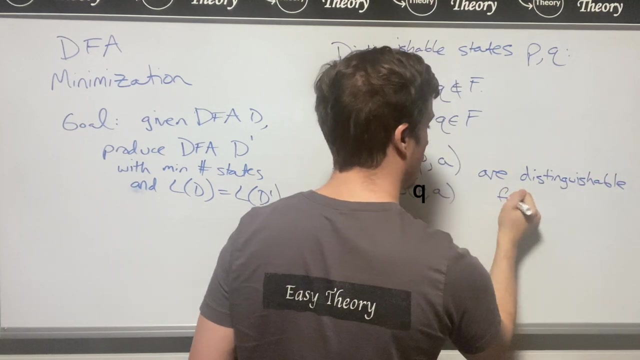 call it A. So look, the same character in both cases. So if it's the case that these two, wherever those two transitions ended up, are distinguishable, So if the result after reading one character for some character A, then that means that these two 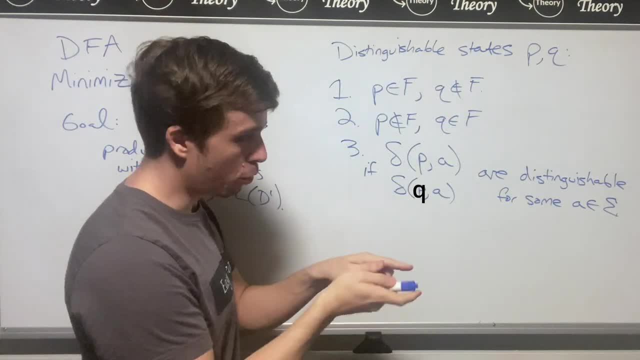 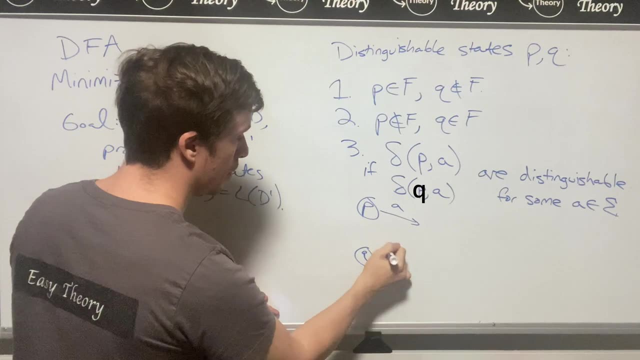 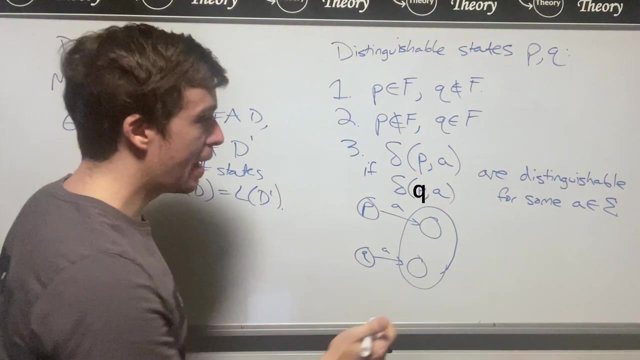 states P and Q are distinguishable Because, wherever they ended up, let's take a look at what that would look like. So P on A goes somewhere, Q on A goes somewhere And we don't know the status of both of these states. Then if these two are distinguishable, then that means 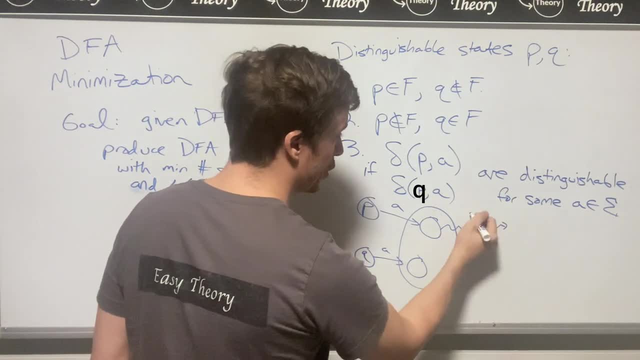 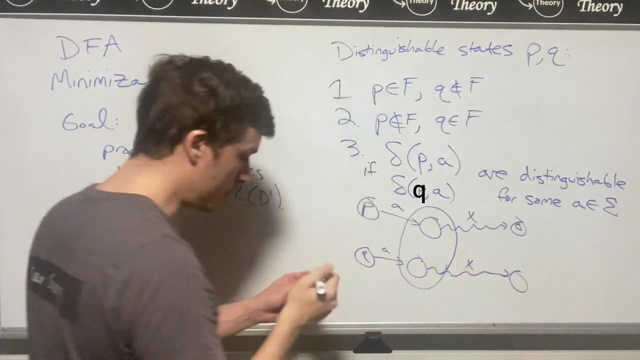 that there's some string- I don't know what it is, let's call it X- such that one goes to an accept state and one of them goes to a non-accept state, Then that means from P and Q's perspective, if we 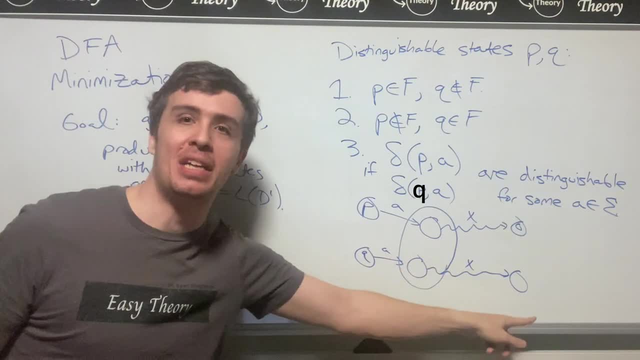 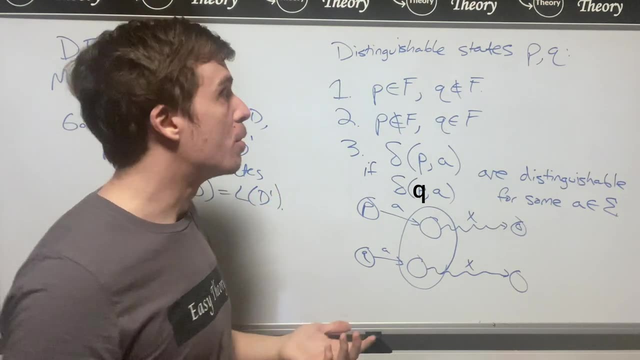 read AX, then one's going to be accepted and one's not going to be accepted. So, therefore, we can actually define this recursively, which is pretty dang cool. All that we're going to do is we're going to make a table that is going to keep track of these distinguishable pairs, So we're going to 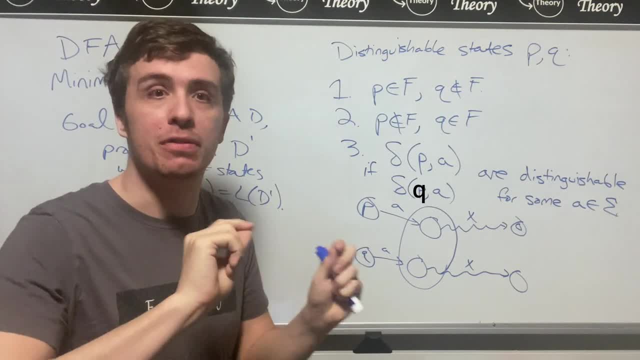 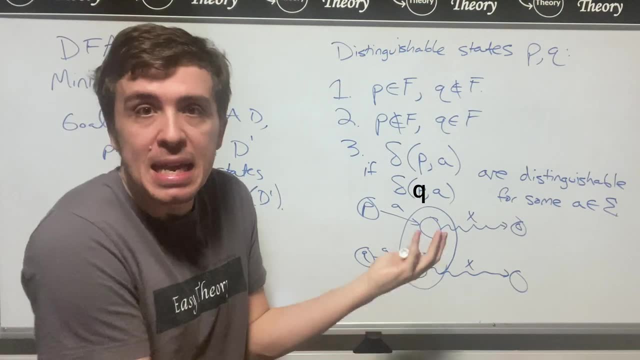 make a table that has two pairs of states. So this table is going to represent pairs of states that we find out are distinguishable And then, at the end of the algorithm, if we haven't found any additional pairs of states, then therefore those two states are indistinguishable and can be. 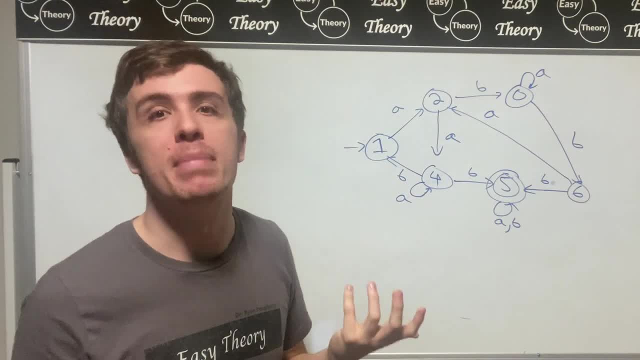 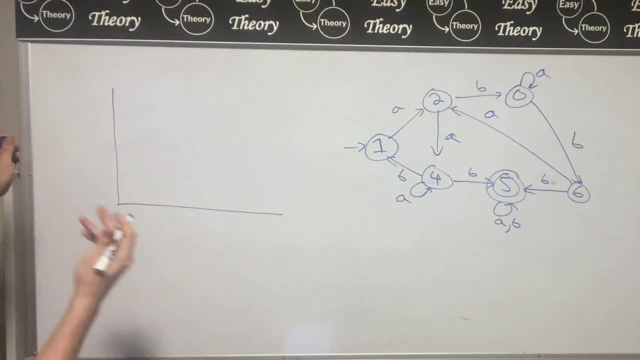 merged. Okay, I made this little DFA right here. Let's try to find the minimum size DFA for it. So what I'm going to do is I'm going to make a little table here, which I'm going to call an AX table, which is going to be looking like this. So I'm going to have a 6x6 table. So I forgot to. 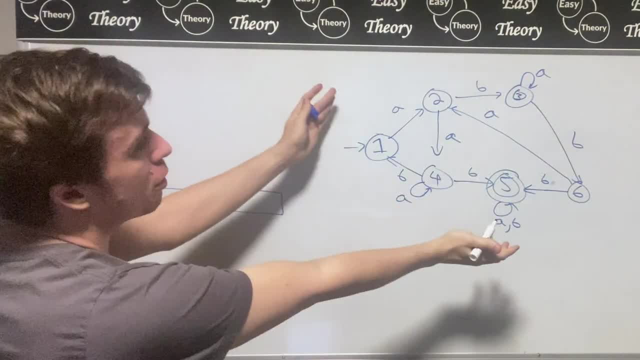 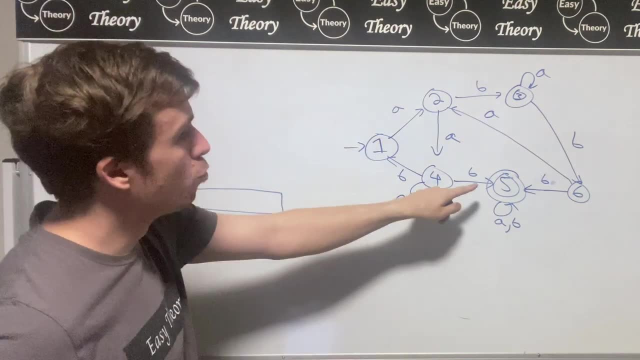 put a 3 here, but I'm going to have a 6x6 table because there are six states here And I'm going to put false in the pairs of states where one of them is a final state and one of them is not a. 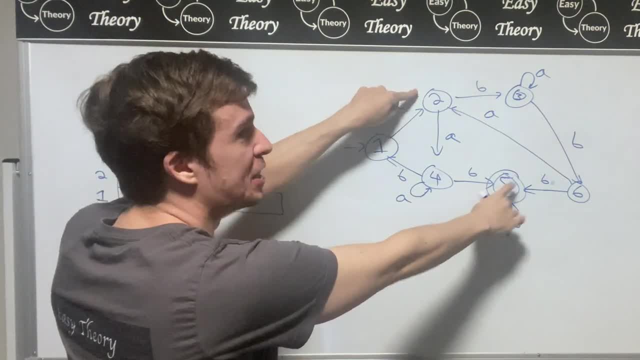 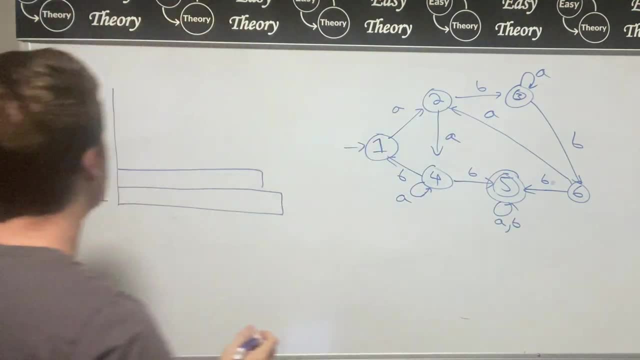 final state. So if I have 2 and 5 being distinguishable, then it's the same as 5 and 2 being distinguishable because it doesn't matter. So I'm going to put false in the pairs of states because it doesn't matter the order, because you're just looking at pairs of states. So what? 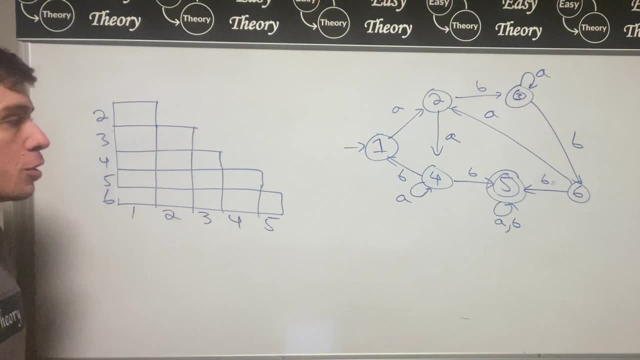 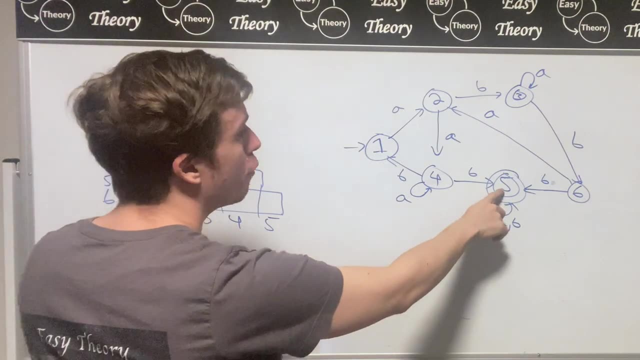 I'm going to do is only have half of the table here, Okay, so here's the initial table. I haven't put the pairs of states, where one is final and one is not yet, So let's look at that. So 5 is going. 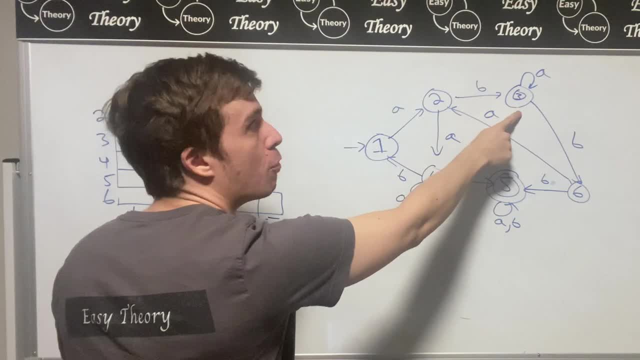 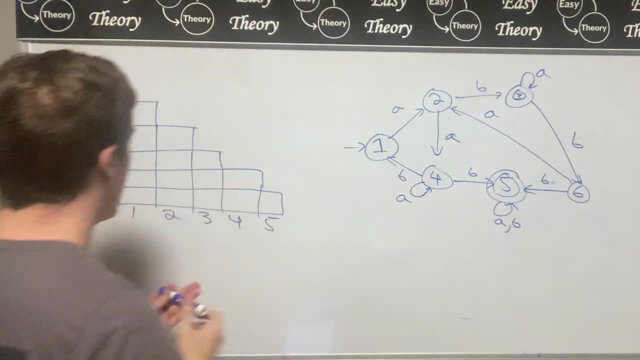 to be distinguishable with every single state except for 3, because it's also a final state. It might be distinguishable later but it's not right now. So 5 and 1, that's going to be marked as distinguishable. 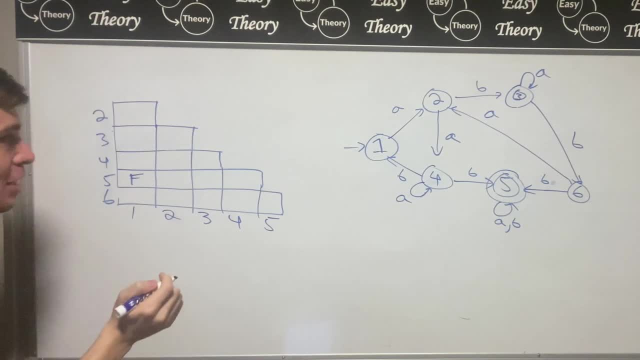 I'm going to mark as F for false that they're not indistinguishable. Then 5 and 2, that's going to be marked as false. So that's 5 and 2 here. 5 and 4, that's going to be marked as false. And 5 and. 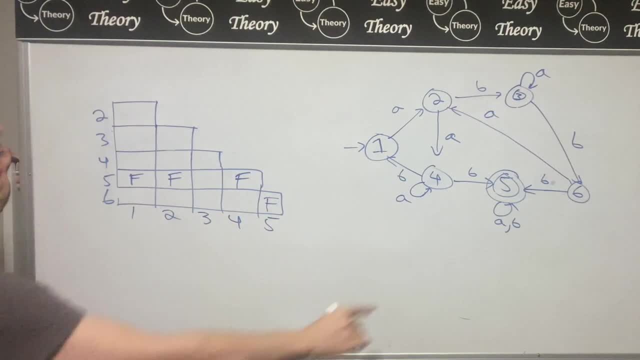 6, which is going to be right here. I'm going to mark that as false too. And then the same deal goes with 3. It's going to be distinguishable with everything except for 5.. So 3 and 1, that's. 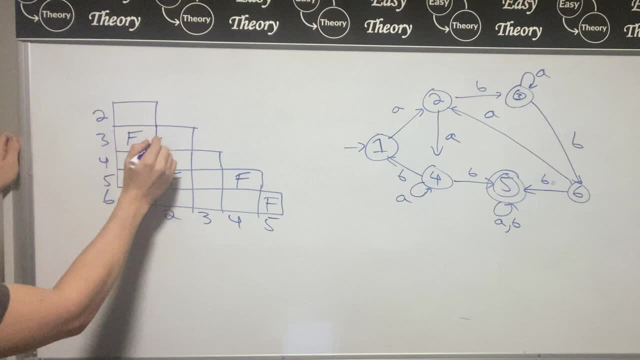 going to be marked as false. 3 and 2 is going to be marked as false. 3 and 4, which is right here, that's going to be marked as false, And 3 and 6 is going to be marked as false. We have no idea whether or not the other things are going to be F yet, but all. 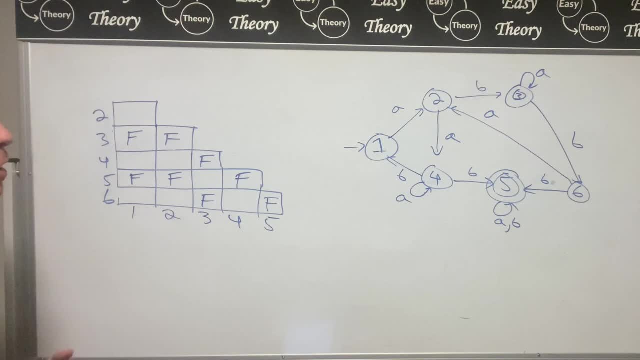 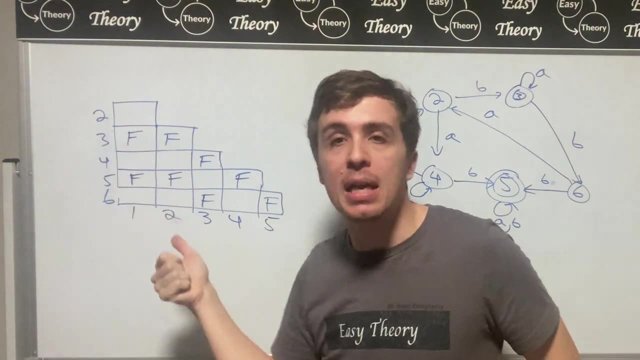 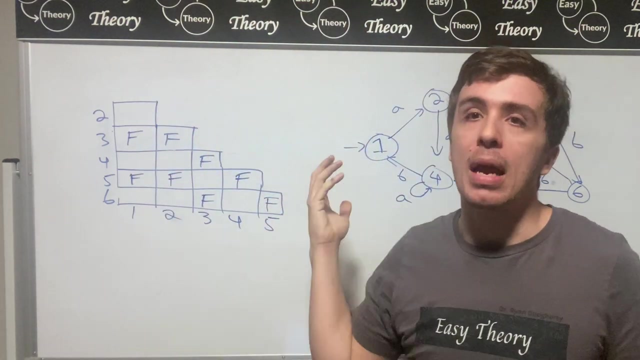 of these things are automatically Fs, So therefore they cannot be merged. So then, now, all the algorithm is is to look at each one of these blank spots and check recursively whether or not the pair is distinguishable. And if we go through the entire table and don't think about the 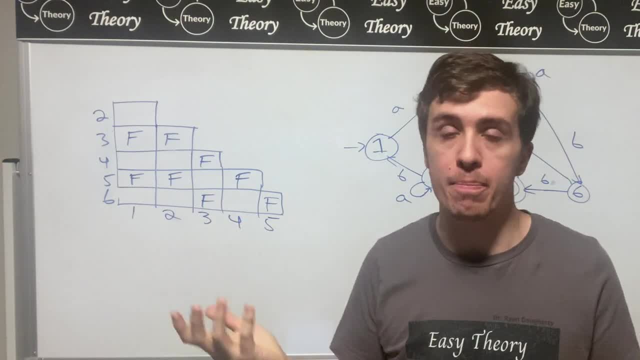 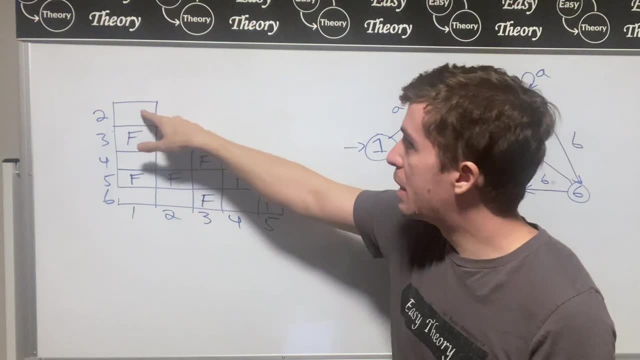 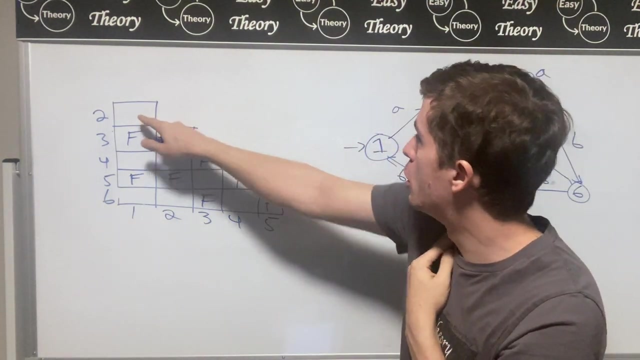 pair, then we're done, because there's no point in going through again. And then everything that at the very end let's just say we have this. then that means that all of these states can be merged together, which is pretty cool. So now let's look at each one of these entries: 1 and 2.. 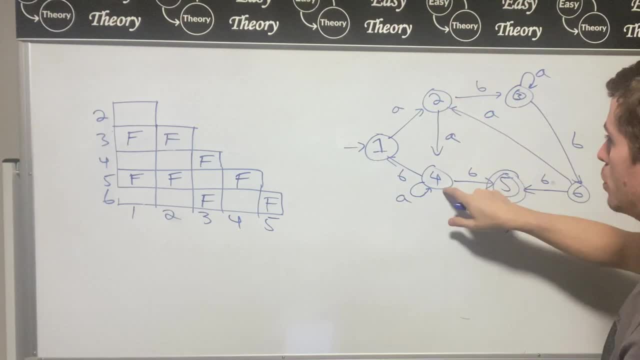 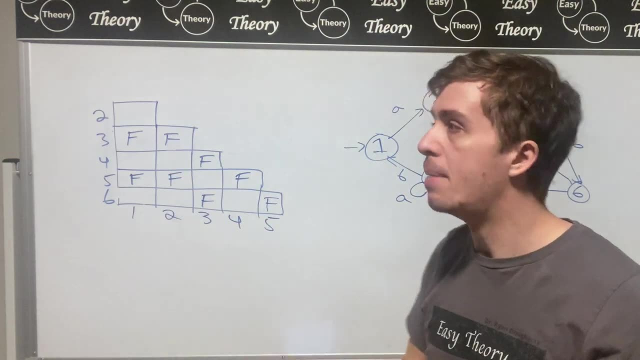 So if we look at 1 and 2 here, let's see where they go on A, So 2 goes to 4, 1 goes to 2.. And if I look in the table, 2 and 4 is not marked, so I don't do anything yet. So then now let's look at: 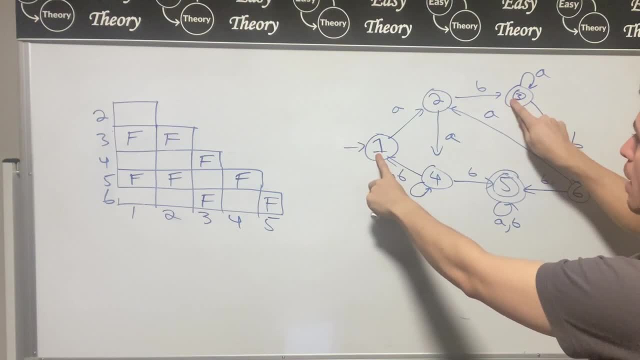 B. So 2 goes to 3 on B and 1 goes to. I actually made a little bit of a mistake here. This needs to go here. 1 needs to go to 4 on B. So then now let's look at what 1 and 2 do. So 2 goes to 3,. 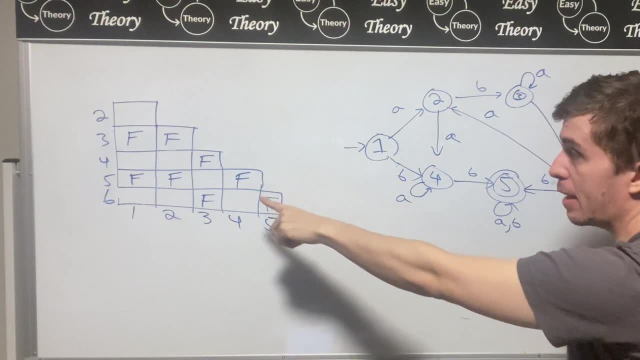 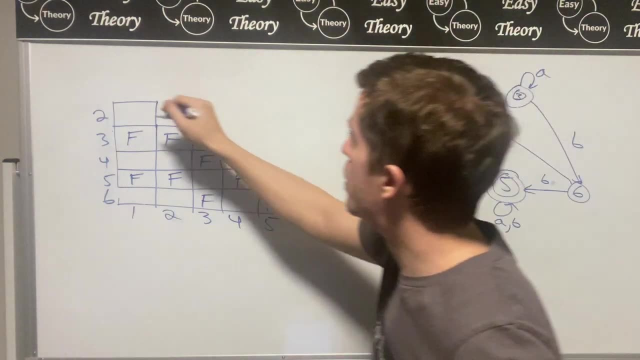 1 goes to 4, and 3, 4 is marked in here. So then, therefore, I'm going to mark 1 and 2 as being distinguished by B, So therefore I'm going to put an F here, Now that we've marked an entry. 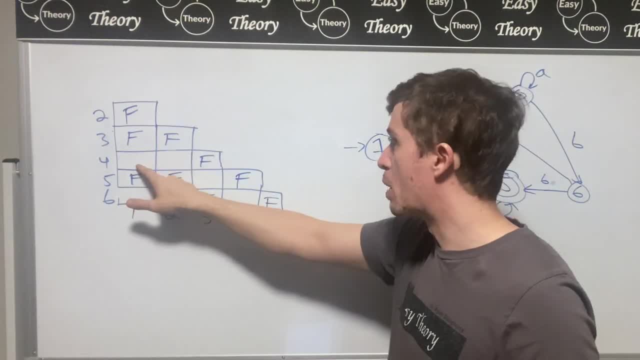 we must go to B. So now that we've marked an entry, we must go to B. So now let's look at another iteration later, but let's keep going. So 1 and 4, let's see: So 1 and 4. on A, let's say: 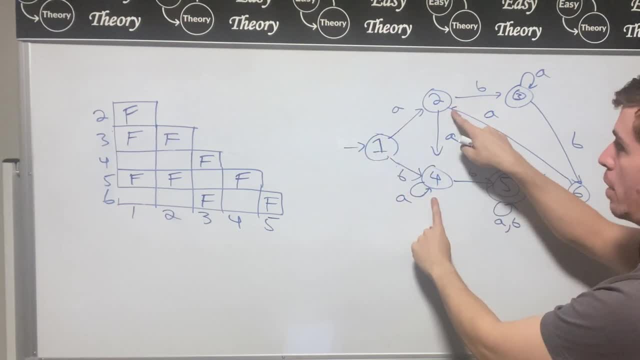 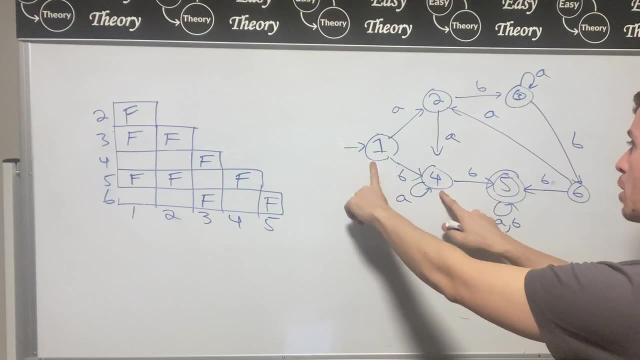 are going to 2 and 4.. So, therefore, and that thing is not marked yet, So that's okay, Let's look at B. So B is going to go to 4 and 5, and that clearly isn't going to be marked. I don't even need to. 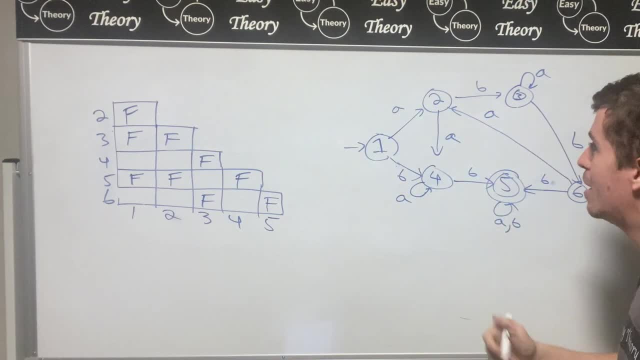 look at the table. There are different parodies of final and non-final. So therefore, 1 and 4, that's going to be marked. Let's look at 2 and 4.. So 2 and 4 on A, those are going to go to 4. 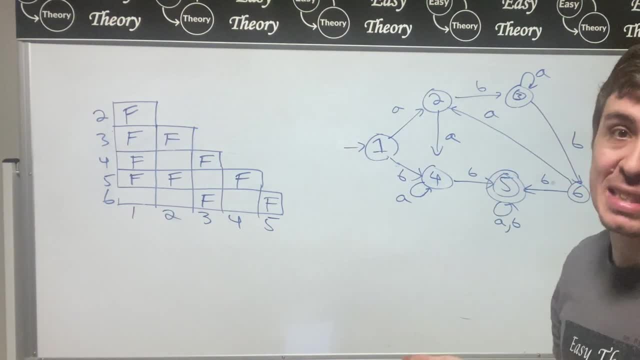 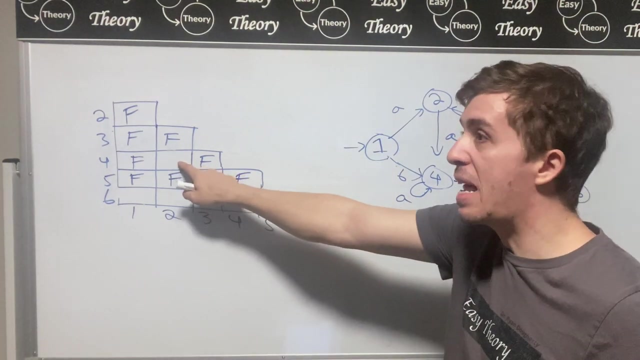 each and then a state is always indistinguishable with itself, So therefore that cannot possibly mark anything. And then, if we look at B, they go to 3 and 5, and those are not marked yet. Mainly, this entry is not an F yet, so I do nothing with that entry, with 2 and 4.. 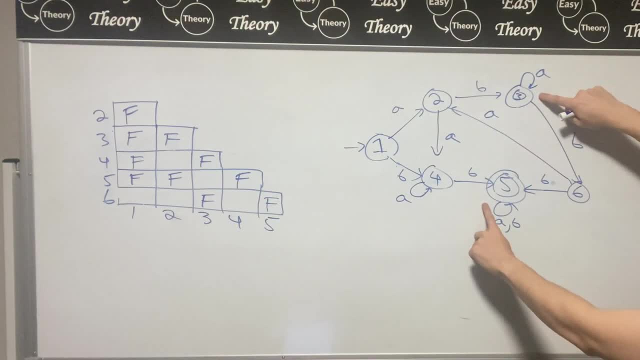 So let's look at 3 and 5.. 3 and 5, input of A goes to itself, and that obviously doesn't change anything. If we look at B, that's going to go to 5 and 6, and then therefore those are distinguishable. So therefore, 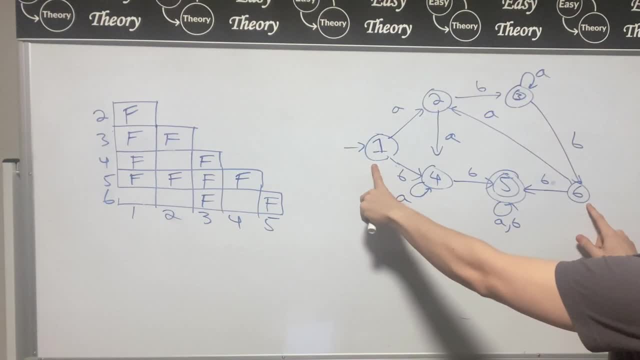 I do mark 3 and 5.. All right, so now let's look at 1 and 6.. So 1 and 6 on A go to the 2 state, so therefore they're the same on that particular thing, And then on B they're going to go to 4. 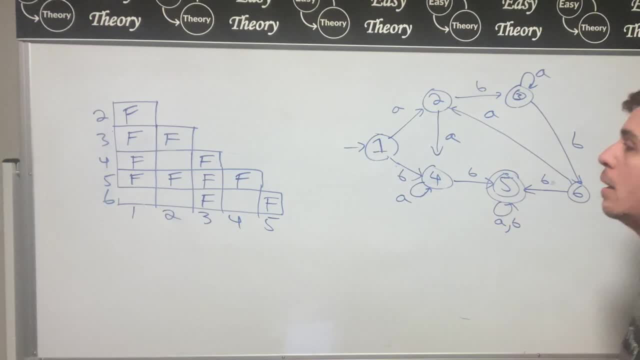 and 5, and then those are distinguishable. I can just look at it. So, therefore, 1 and 6 is going to be marked. Let's look at 2 and 6.. So, on A, they're going to go to 2 and 4.. 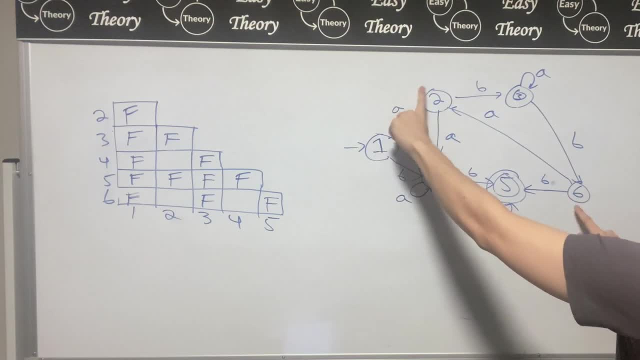 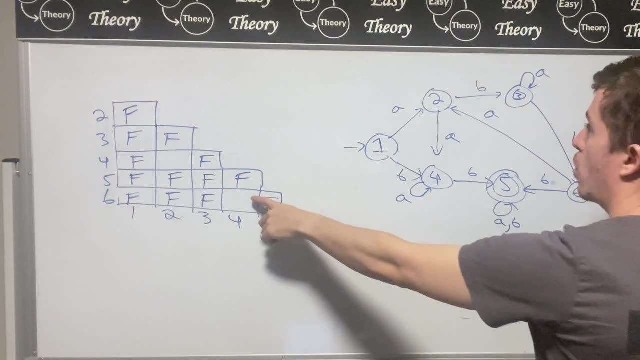 I have not marked that yet. If we look at B, those are going to go to 3 and 5, which we have marked. So therefore, 2 and 6, that's going to be marked. All right, let's look at 4 and 6.. 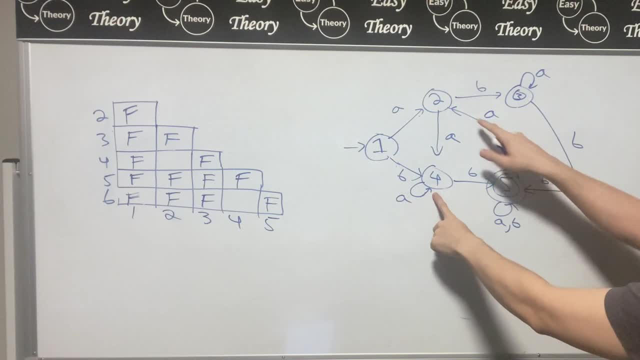 So 4 and 6. on A, those are going to go to 2 and 4, which we have not marked yet, And then on B, they're going to go to the same state and that obviously will never be distinguishable. So we don't have to worry about that. So therefore this is not marked. 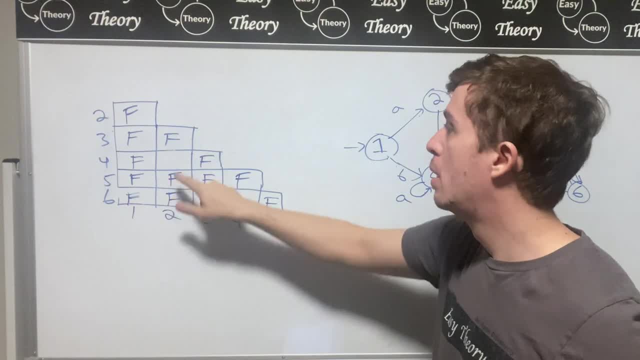 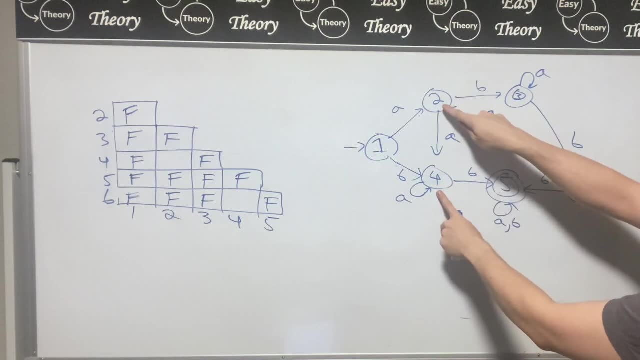 Now let's look at 2 and 4 again. So now this is the second time through- Let's look at 2 and 4.. So 2 and 4? on A they go to the same state, so that's never distinguishable. On B, they're. 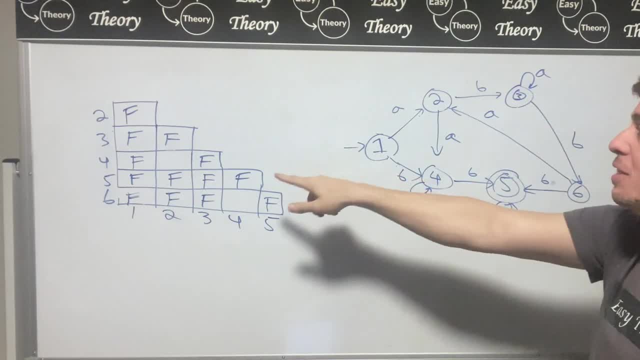 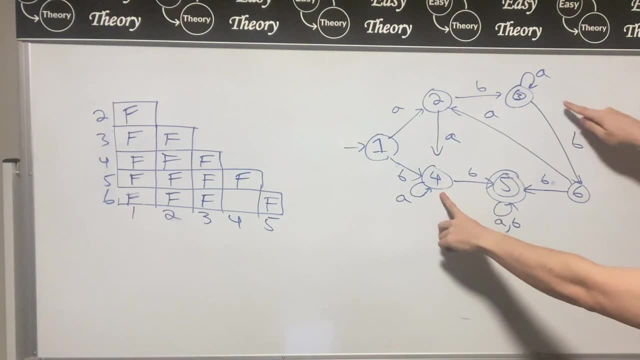 going to go to 3 and 5,, which is distinguishable now, And so therefore I'm going to mark 2 and 4, which is going to be F, And then 4 and 6, we saw on B, on A. sorry, they're going to. 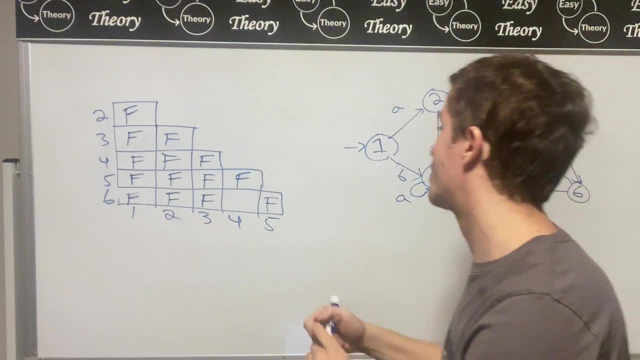 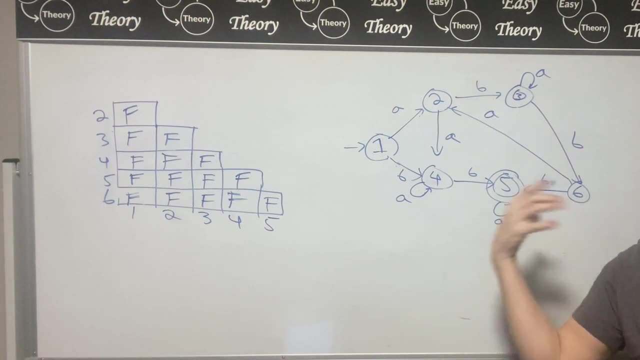 go to 2 and 4, which we know to be distinguishable now, And so therefore, every single entry in here is marked. So therefore, this is the minimum size DFA for whatever language it is. Now let's do a slight variation on this, where I'm going to have the exact same states. 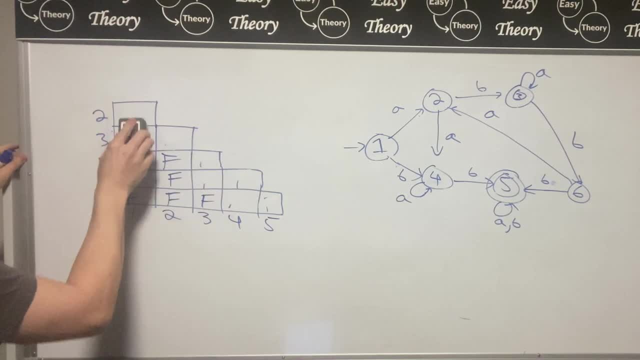 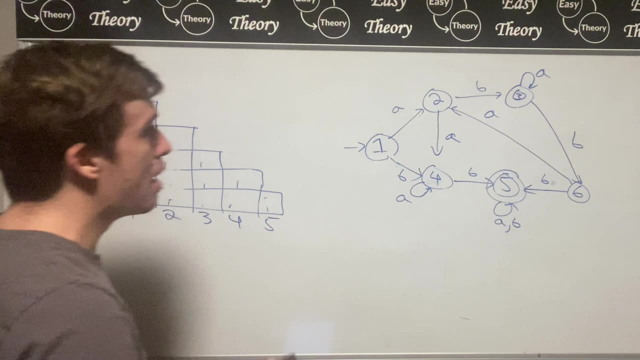 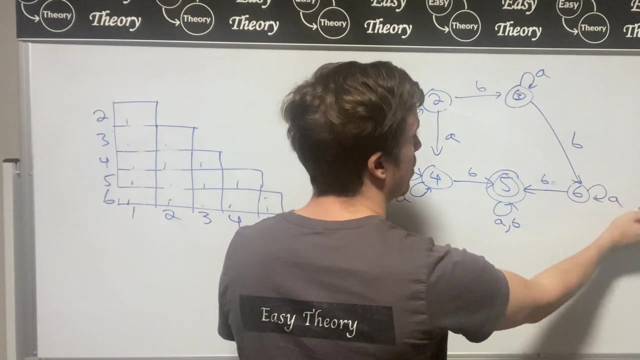 but I'm going to modify the transitions a little bit so that we actually do get a smaller thing. So I'm going to have this table be completely wiped out. But now all I'm going to do is I'm going to have this transition be a self loop on six. this b is going to be a self loop on three. 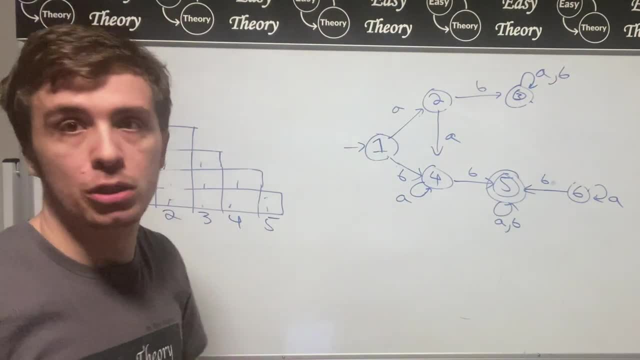 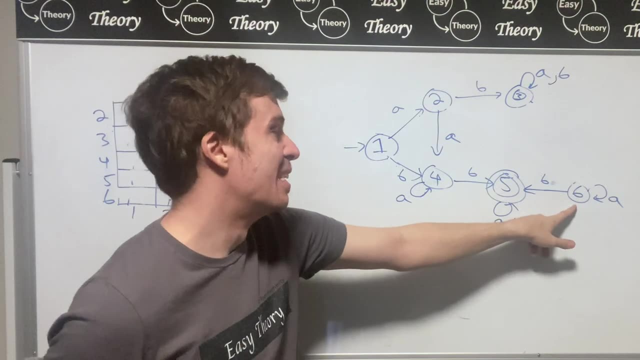 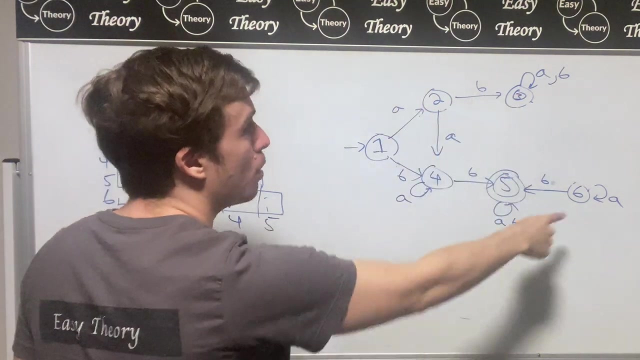 and that's all I'm going to change. it's going to be exactly the same dfa. otherwise, obviously, state six is going to be eliminated because it's uh, not, you can't even get to it. but we'll deal with that, okay, so three is going to be distinguishable with every state except five. 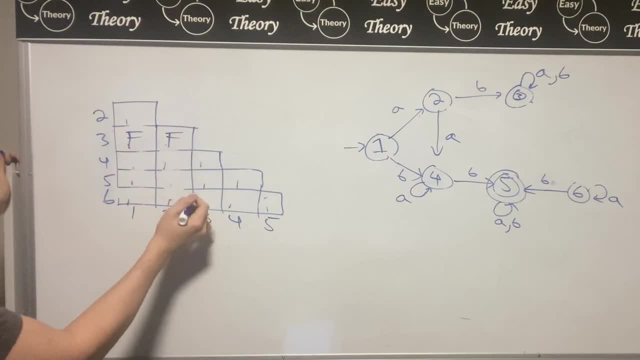 exactly the same as before. so these f's are gonna uh all be in here, so not with state five, we don't know that yet. and state five is going to be exactly the same with every state except for three. so this is an f, this is an f, that's not an f. yet this is an f, that's an f. so then now let's carry. 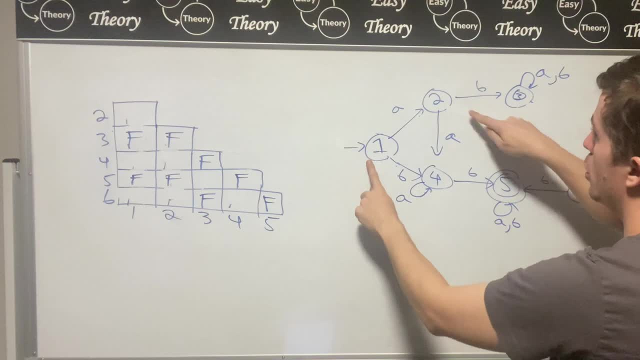 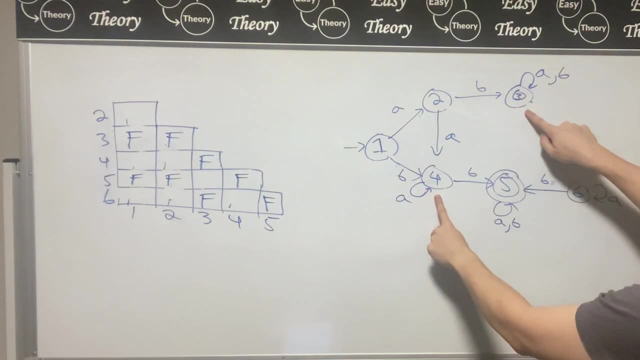 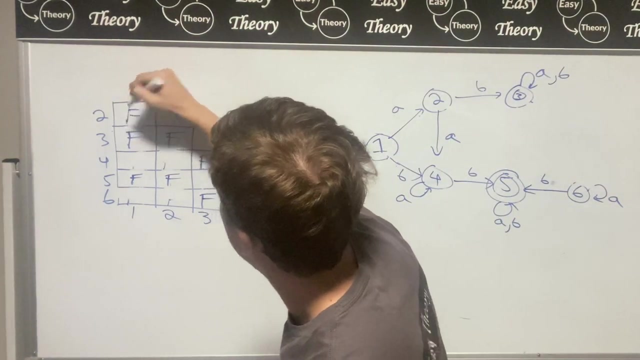 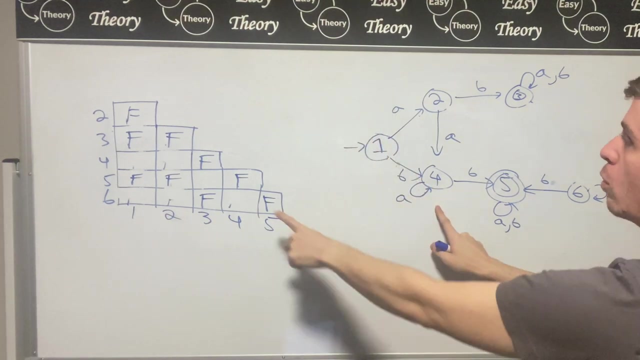 through again. so let's look at each entry: one, two on a, that's going to go to two and four not marked. yet let's look at b, those go to three and four, which is marked, and so therefore I'm going to mark one and two. so that's an f. if we look at now, one and four on a, that's going to go to two and four, which 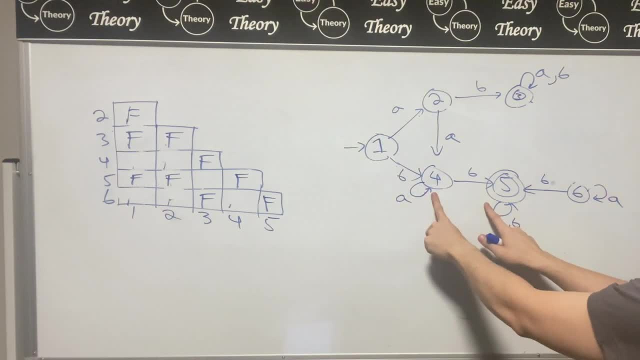 we have not marked yet. if we look at b, that's going to go to four and five, which is marked, so I'm going to mark this here. if we look at two and four on a, again, they go to the same state. that didn't change from before. 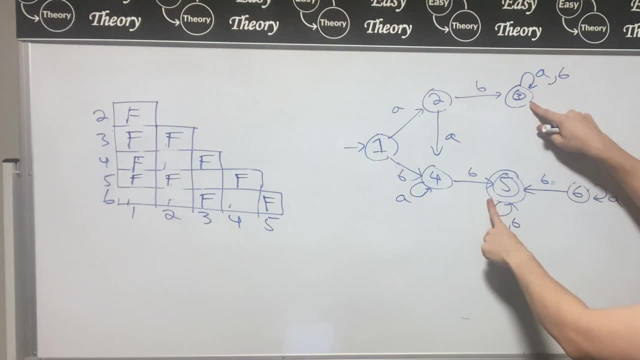 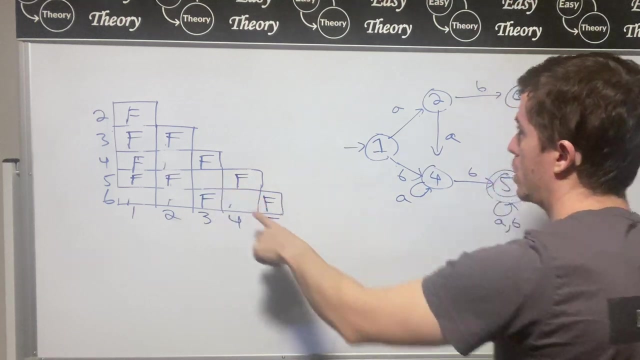 if we go on b, we're going to go to the same parity of states. they're both final and that's not marked yet, so therefore I'm not going to mark two, four just yet. if we look at three and five, they're going to go to the same pair of states. so this entry is actually never going to be marked because 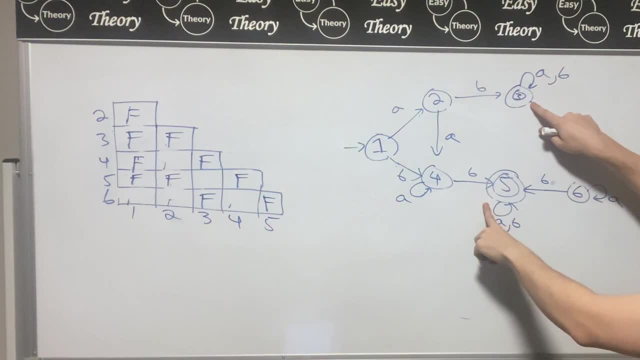 it's a dfa. I'm never going to get out of these states once I enter them, so therefore this entry will never be marked. and then therefore we know we can contract these, but I'm not going to do that yet if we look at one and six. so therefore, on a, that goes to two and six, which is not marked, on b, they 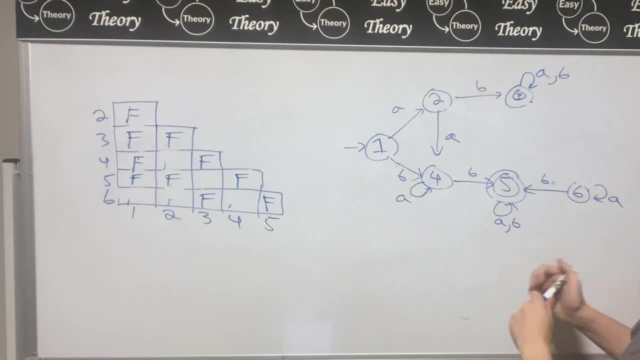 go to four and five, which we know to be marked, and so, therefore, these states are indistinguishable because they go to a pair of states that's marked. if we go to two and six, that on a is going to go to four and six, which we know, which is not marked yet on b, that's going to go to three and five. 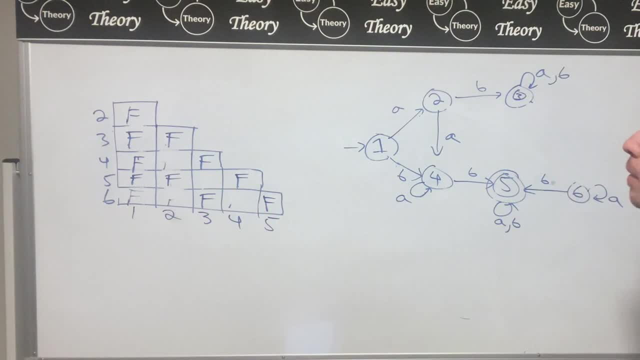 which is not marked. so two and six can't be marked. yet if we go to four or six on a, they go to themselves, which won't change anything. if they go to b, that will never change anything. so actually, four and six is never going to be marked either. so let's go through. 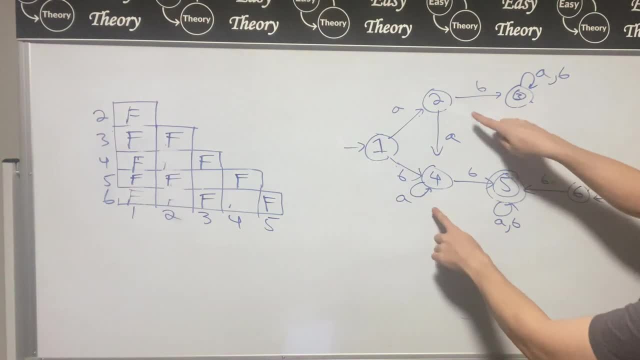 another iteration: uh, two, four, two, four. on a, on input a, that doesn't do anything. on b, that goes to three, five, not marked yet, so that doesn't do anything. three and five will never be marked. two and six, that goes to a, four and six, which is not marked. on b, they go to three and five, which is. 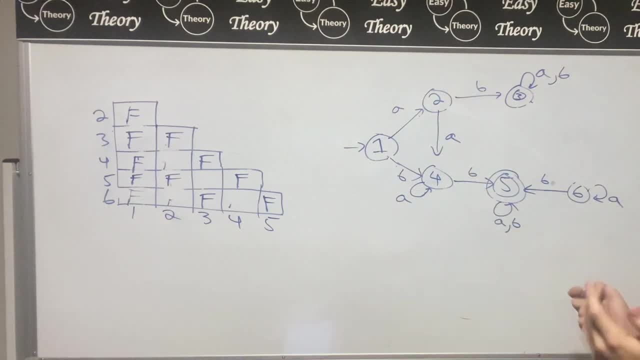 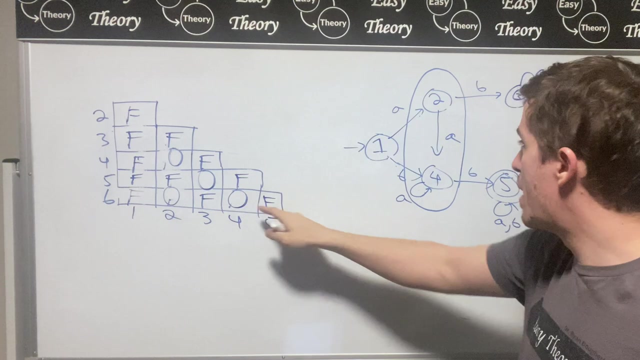 never going to be marked, and four, six we've already determined will never be marked. so these four entries represent indistinguishable states. so therefore four and two can be merged. so what we can do is we can treat this as one state. uh, in fact we can even put six into the mix. 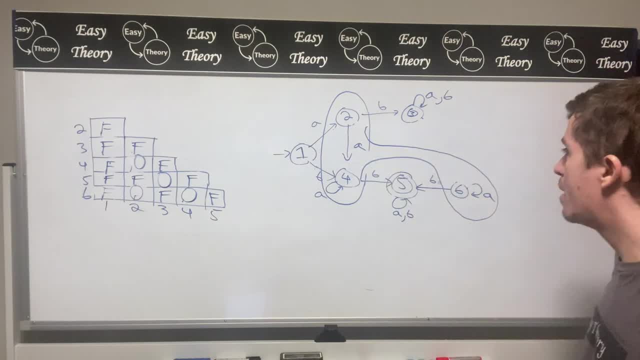 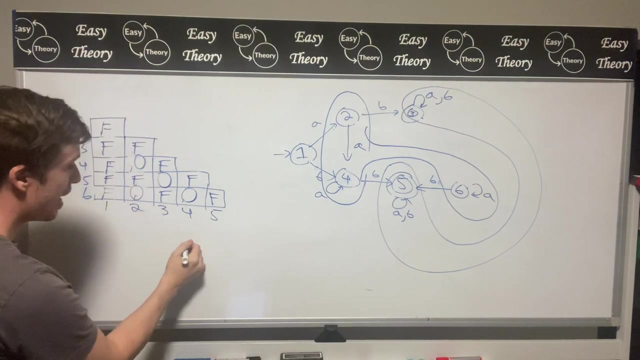 that rhymes, so we can have it be looked like that. so that's one state right now, and we can have five, and three represent another state. so I know that the figure looks a little complicated. so so once you do all of the reducing here, what you get is something that looks like this: so you get state one that 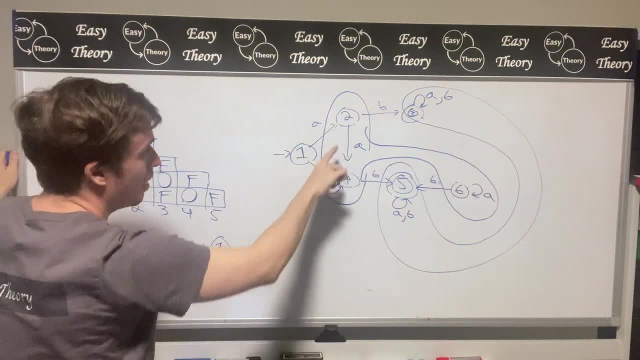 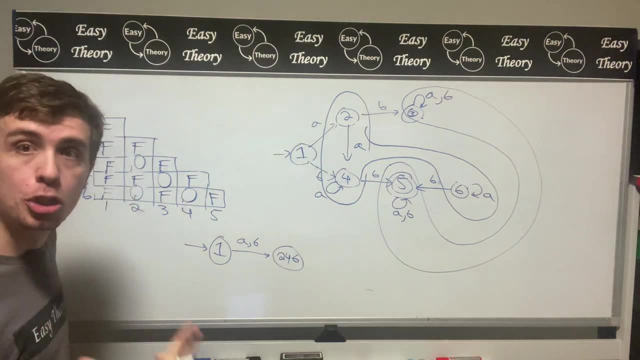 goes to on a and b, to this three state Hydra thing. so on a and b, that goes to a state I'm going to call two, four and six, that's going to represent states two, four and six, and then that self loops on a so that if you're in 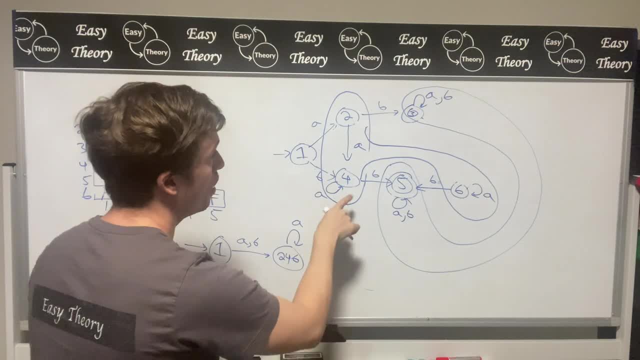 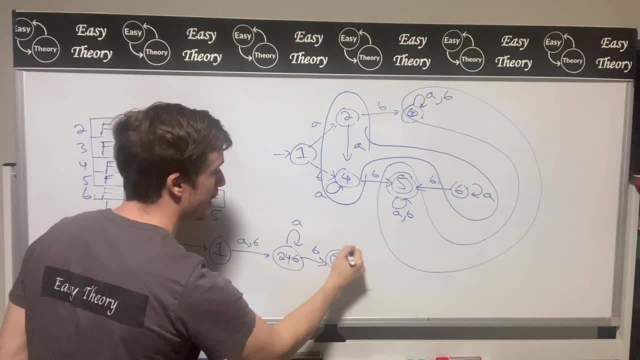 this bubble, right here, if you read an- a, you're going to stay within the bubble and if you read a- b, you're going to go to the three, five bubbles. so therefore, on b, they're going to go to a final state which is going to self-loop on everything. because in this bubble if you read an a or a b, 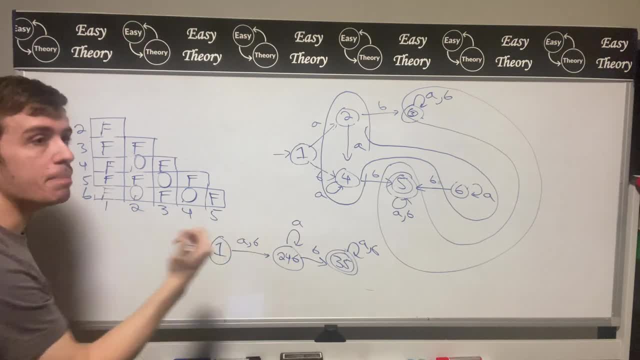 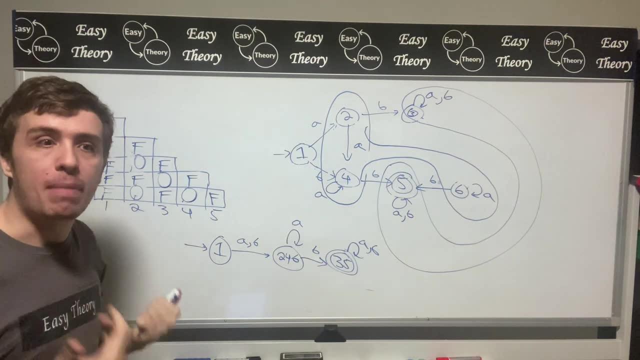 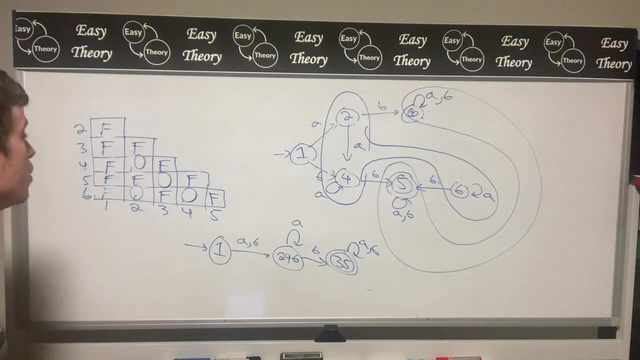 you're going to stay within the bubble and then therefore, this is a minimum size DFA for this particular language is the minimum size DFA requires the my hill and the road equivalence relation, which I have proven on the channel before, but I'm not going to prove here. all that you need to know is to make a little. 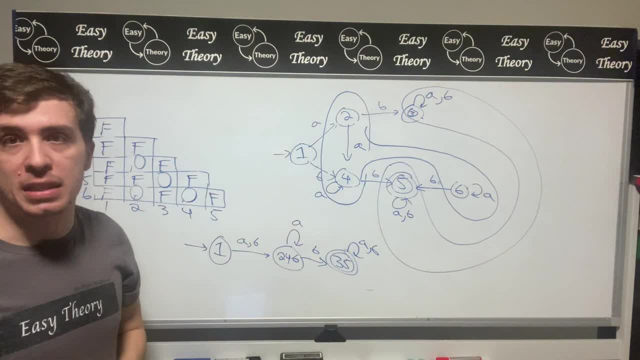 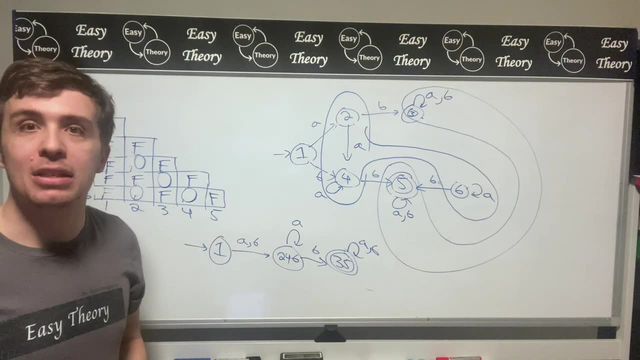 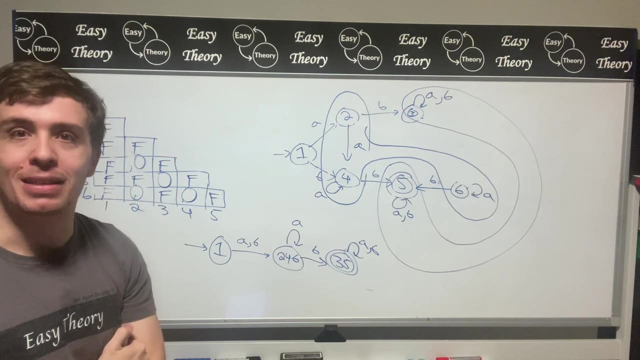 table like this and then just carry out the procedure as I described and then, therefore, you will get the minimum size and unique DFA for that language. so hopefully that was interesting. leave thoughts about the DFA minimization algorithm into the comments down below. as always, please like the video and subscribe to the channel. it really helps. 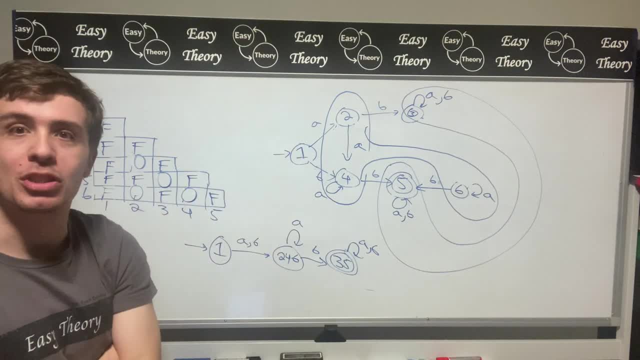 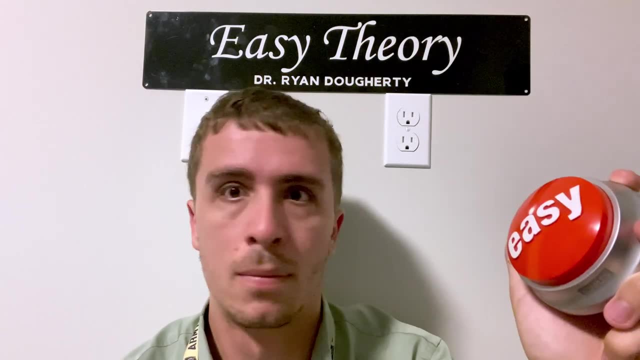 us out. there are many other links in the video description if you want to support the channel further. and, as always, thanks for watching and I'll see you next time. that was easy. that was easy.